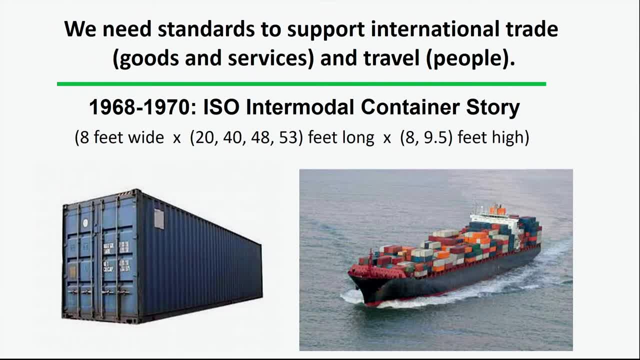 So why are standards important? And basically, standards exist, at least at the international level, to promote international trade and travel. The best example, as shown on this slide, is that after the Second World War, there were a number of efforts developed to foster trade, And at that time trade consisted of products that were put on pallets and loaded. 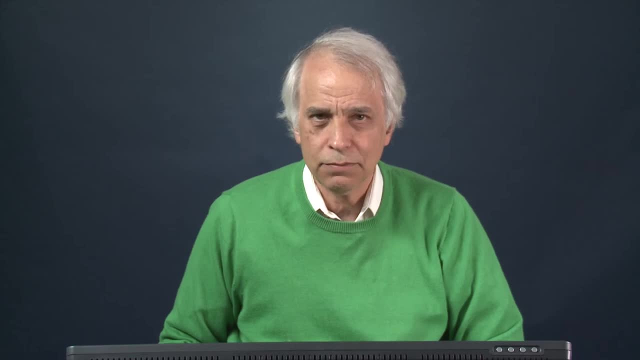 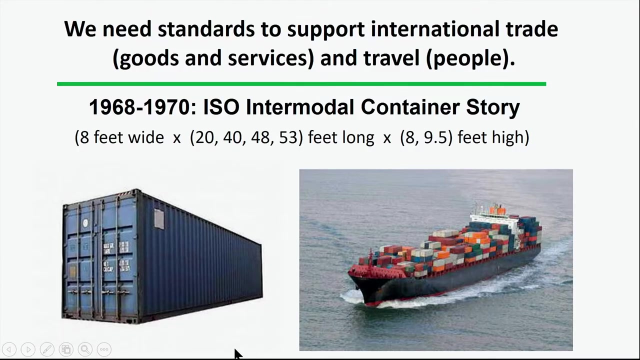 onto ships and moved internationally. The difficulty was that there was a lot of pilferage at the docks, that loading time took a long time because it was individual pallets and so forth. So what was developed, as shown on this slide, is the international standard container. 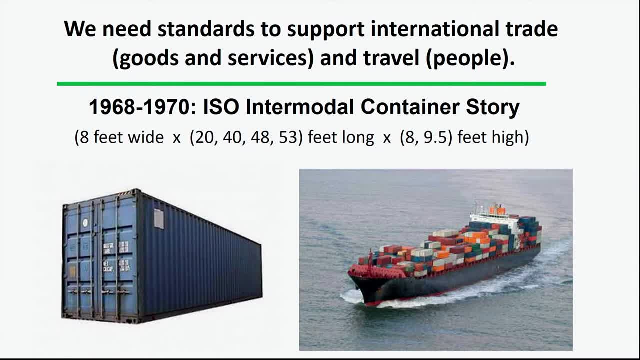 Now the difficult part is the container needed to be interfaced with a wide variety of items. It needed to fit on trucks, It needed to fit on rail cars, It needed to fit on ships, It needed to be handled by cranes, And all of those had to be designed in such a way. 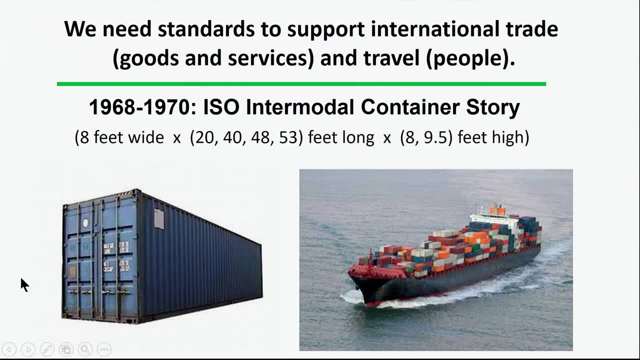 that they would all be compatible with the container shown here. And if none of those items was compatible with the container, then international shipment would not happen. And, as we know, once the container came around, then international trade boomed because it was just much easier to do. 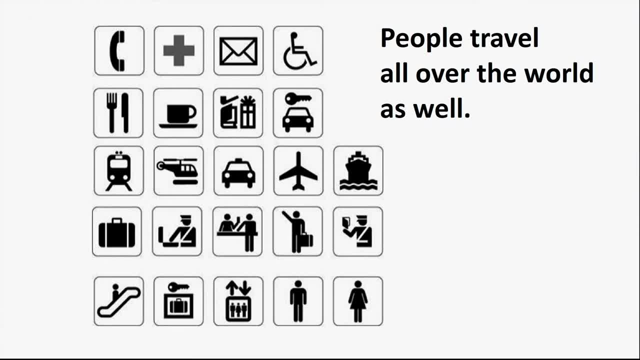 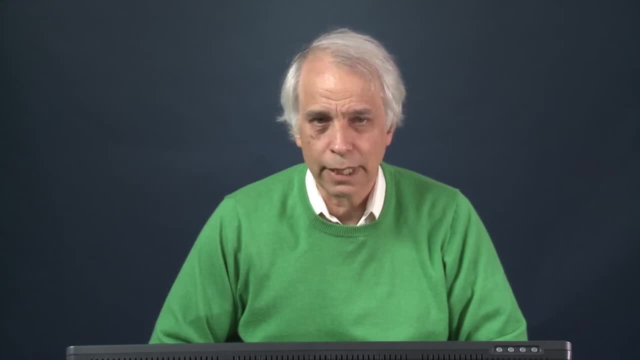 And safer and more reliable. Second point is international travel is important. People travel all over the world. Here's examples of symbols that you might find in an airport or a train station And clearly, if you're in a country where you don't speak the language you'd still need to be able to move around. 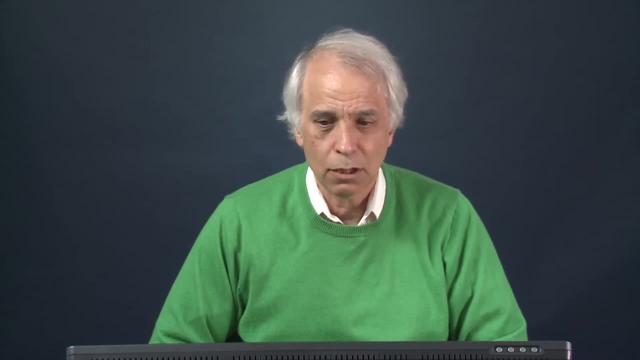 And having symbols as opposed to words, where you don't know the language, overcomes that problem. So I want to talk about standards-related documents, And they have a number of names and they vary And they're in a variety of dimensions. So, first of all, standards can be grouped into: 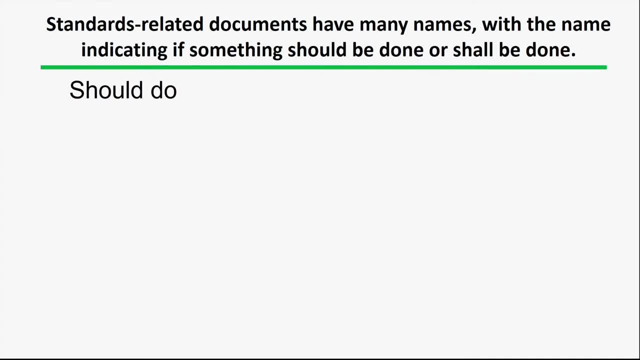 two broad categories: One that describes what you should do, So, for example, we might have guides or guidelines or information, reports or a variety of names that use the word practice, Best practice, code of practice, consensus practice, recommended practice And the same. 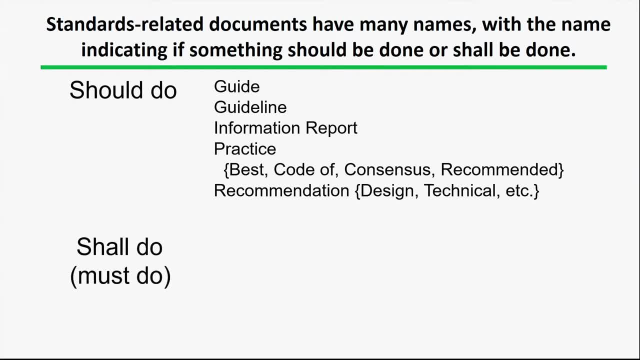 thing is true for recommendations. In addition, there are documents that exist that say what shall be done or what you must do, And those include a variety of laws, regulations of various types, rules, specifications and standards. And what I want to emphasize is, although there are these two broad categories, 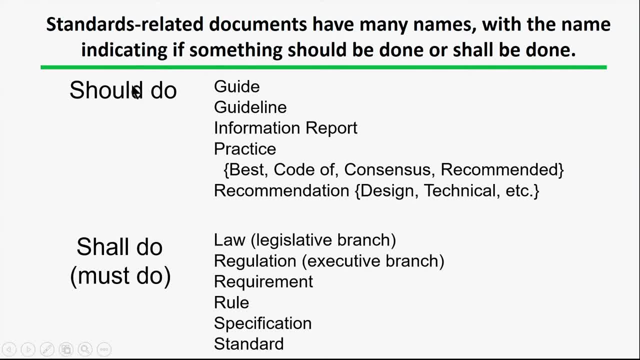 that sometimes something like a guideline, which is in the should case, has in it parts that are regarding what shall one do, And there are other times there are documents, like laws, that might sometimes just say what you should do. So it's not as if a document 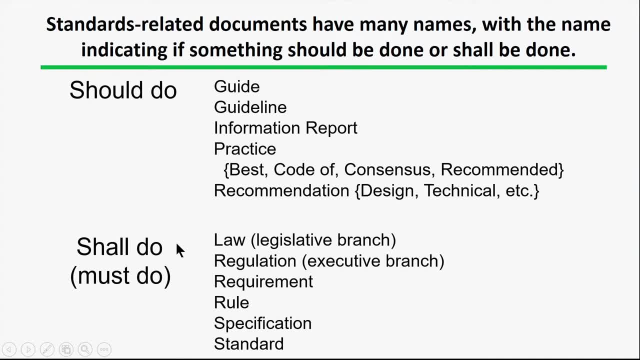 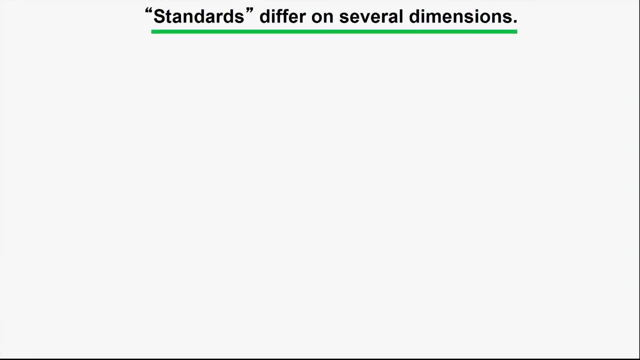 in one of these categories is strictly only shoulds or strictly only shalls, but there tends to be sometimes a little bit of a mixture. So in what ways do standards differ, What's in them And how do we think about them? So the first issue that's important is: who creates it? Is it a government agency? Is 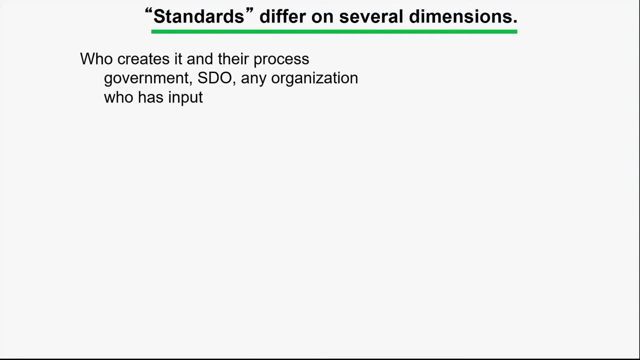 a standards development organization, commonly referred to as an SDO Or some other organization, and who has input into the process. For trade associations and others, input is only for members of the trade association. For standards development organizations and government organizations, input is from the public. 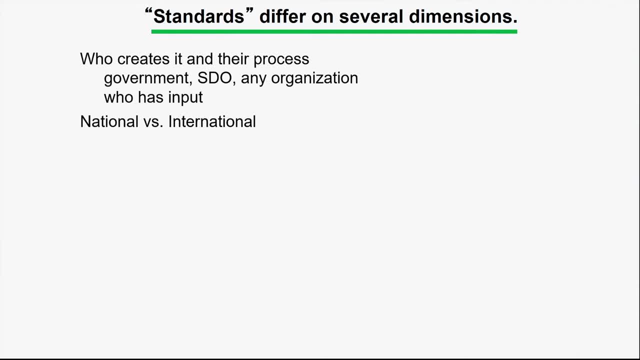 Second is: what's the breadth of the application? Is it a national standard, or within a particular country, or an international standard? Is the document available publicly? Is it some sort of trade secret, or is it an international standard, an ISO standard or something else put out by a public standards organization? 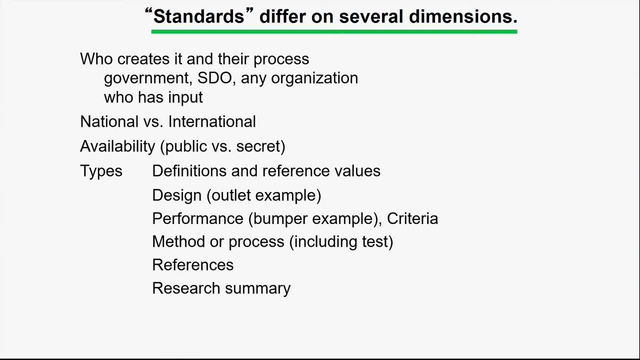 And finally, these documents differ in the kinds that they are. So there's some and some. many standards have a mixture of a variety of types in them, But typical parts include definitions and reference values. You know how is this term defined- Design? So, as shown here, here's an outlet and there might be a. 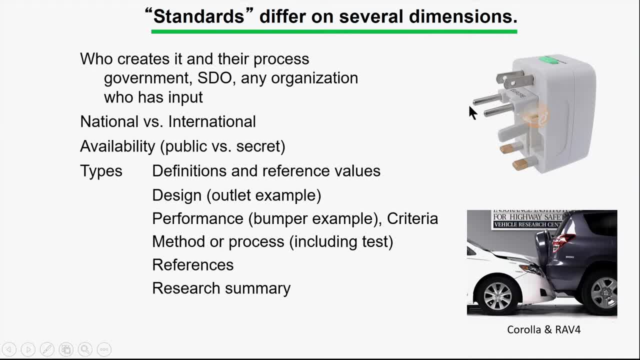 specification for this part, this adapter, and the spacing of these pins, the diameter of these pins, etc. will be specified. in order for one to be able to plug into an outlet, The plug and the outlet have to be consistent, so therefore the dimensions of those parts have to be well defined. Performance: 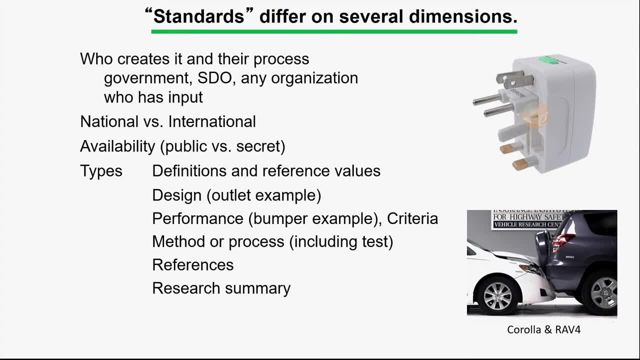 criteria. So here's the case where you can specify not the physical dimensions of an object but how well it does. So one would argue, gee, this is not a very good case for a performance specification because in order for the collision to be avoided, the heights of the two bumpers need to be the same size. 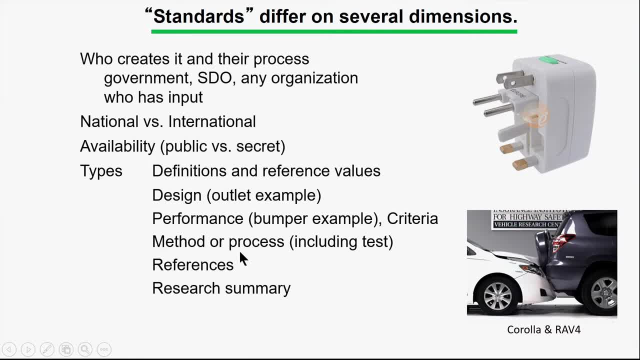 and the same height Processes, examples. So here's a case where you might specify how something is made or verified or checked. There are other standards that are simply lists of references. Normally these are information reports, but they may be for some other purpose. And finally, within this information report, 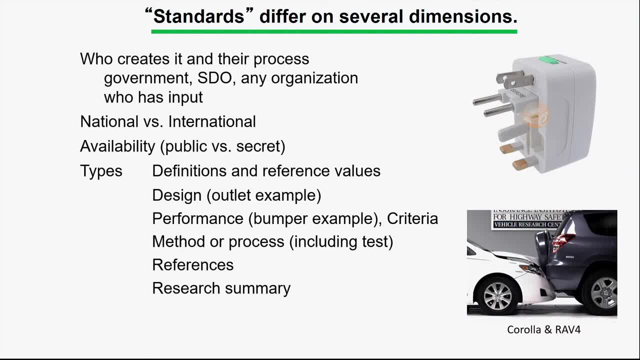 category are standards that really are general summaries of the literature. Last point is again the concept of authority. Does this document give shoulds or shalls in it? And also there's the issue of enforcement. I almost forgot that Enforcement is: are these standards voluntary or required? Now there are some. 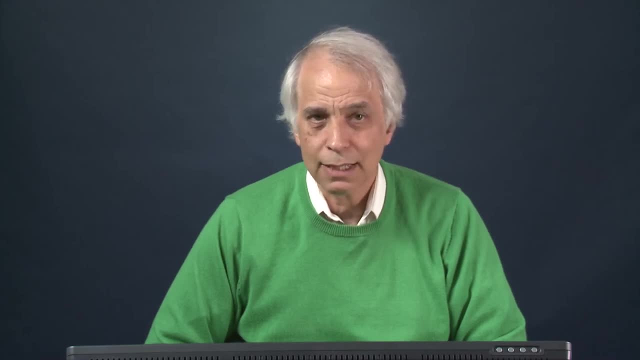 interesting things where what seems to be voluntary is actually required, and that's the case of some international standards where countries will say that in order for a product to be imported into a particular country, it must meet all recognized international standards. So, although international, 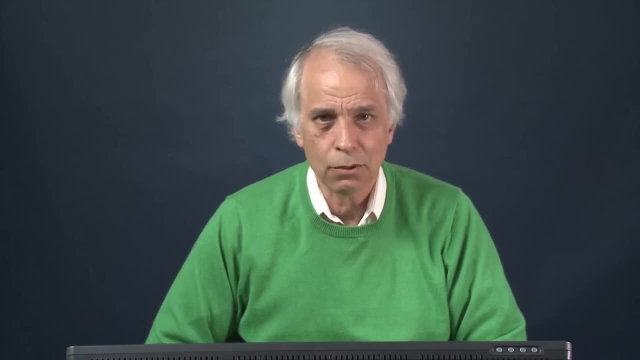 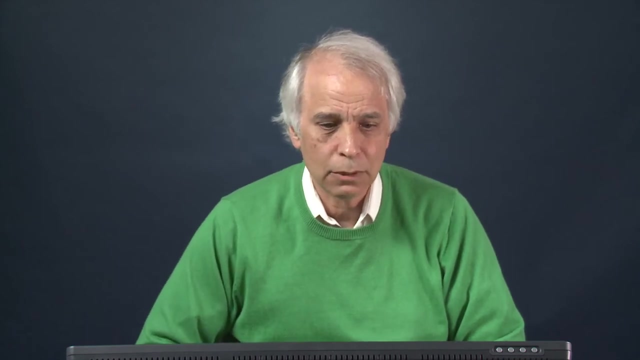 standards such as those from the International Standards Organization, ISO, are voluntary because the country requires it for something to be imported. so-called type approval- that, in fact, was a voluntary standard, then becomes a required standard. What I'd like to do is just talk about one standard as an 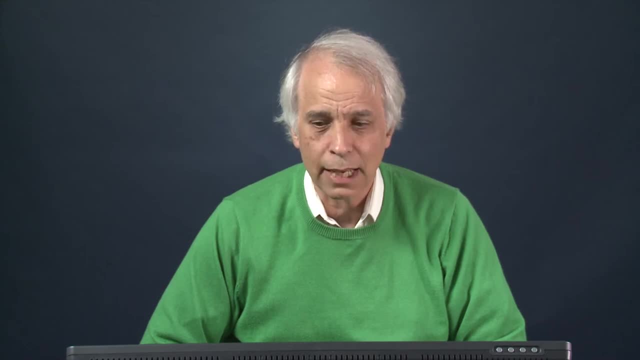 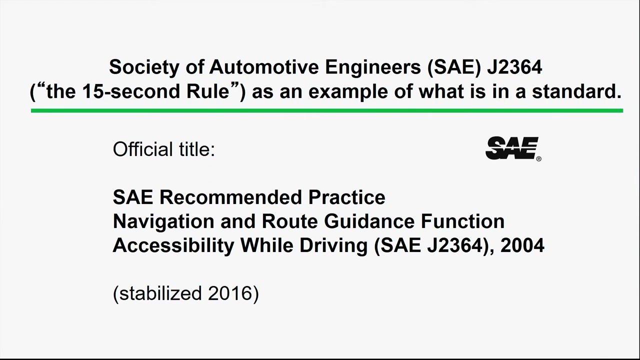 example to give you a sense of what's in them and what they actually say. So the example I want to talk about is SAE J2364, a document that I basically wrote, commonly referred to as the 15-second rule. Now this standard is now stabilized. 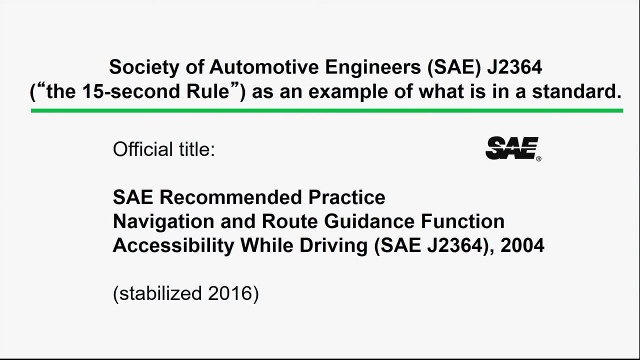 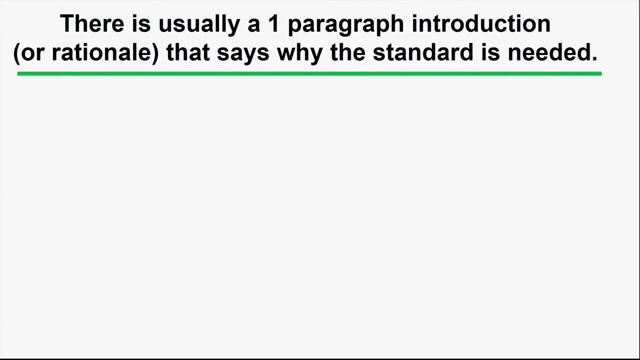 so that no further work is happening on it. but you should know what it's about and just what's in it. So all these documents have a title, as shown here, and the title can be rather technical. Most standards have something at the beginning as an introduction or 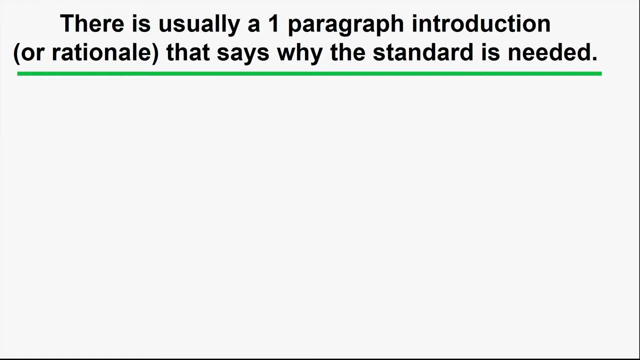 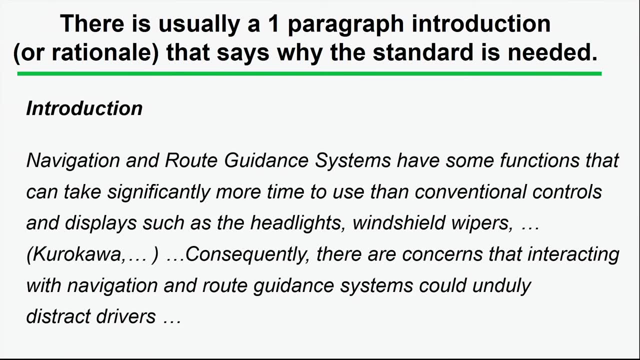 rationale that makes the argument for why the standard is needed. These vary in terms of how effective the arguments really are. For SAE J2364, here's an example of what the introduction is like. So, for example, it makes the argument that it takes more time to operate these functions, so that 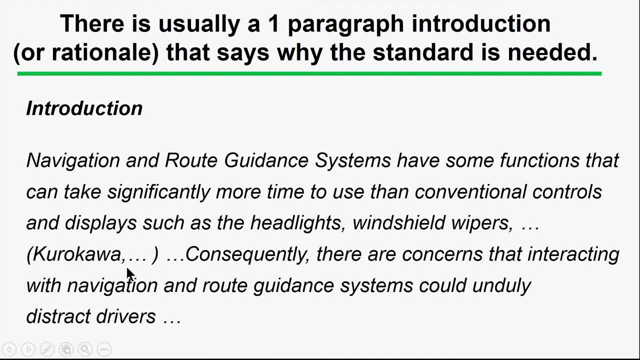 says why one might need such a standard. It provides a citation for that particular information and then talks about further problems associated with this particular issue. and that's the rationale for this kind of document. Again, sometimes the introduction may just provide an overview and a rationale can be a separate section, but it is 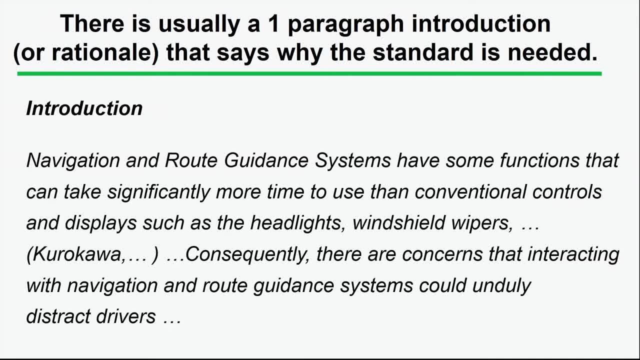 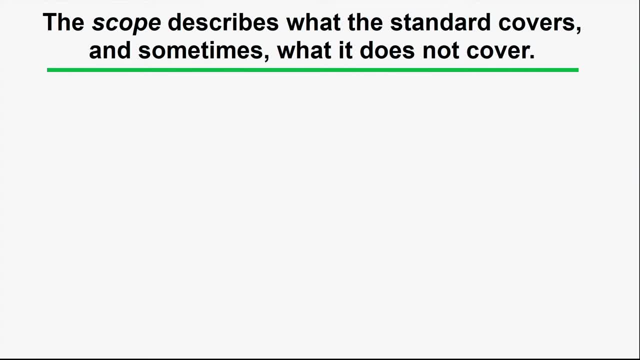 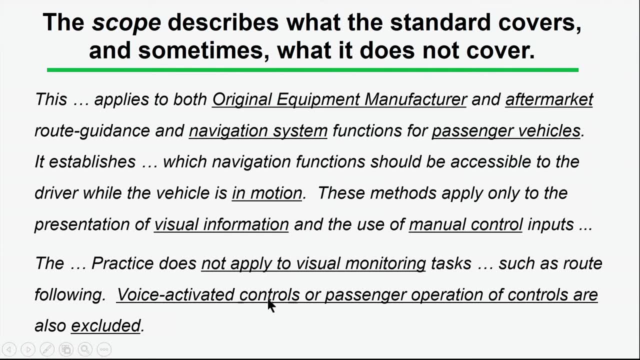 important to have a strong argument for why a particular standard is needed. In this case, it's actually a recommended practice. Also, there's some information that describes the scope, and here's an example of a scope for SAE J2364 to give you some context. So first point is it: 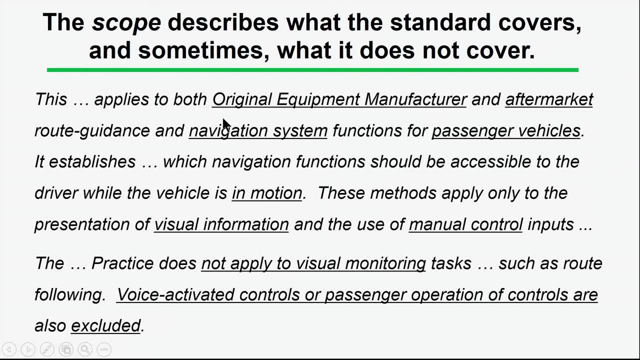 applies to original equipment- meaning that's what the manufacturer who made the product. they have to comply with this- but also aftermarket devices. So, for example, if we're interested in navigation, we're interested both in navigation systems that are built into the car, but also navigation systems that. 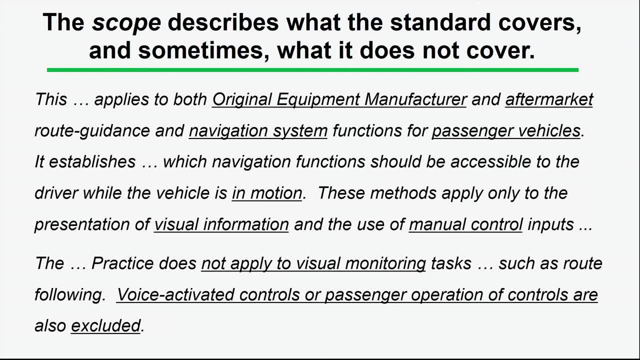 users might play Plug-in or potentially even things that are on their phone. And next point is that the real issue is how the system operates when the vehicle is in motion. Clearly, if the vehicle is parked and you're doing things, there are less safety. 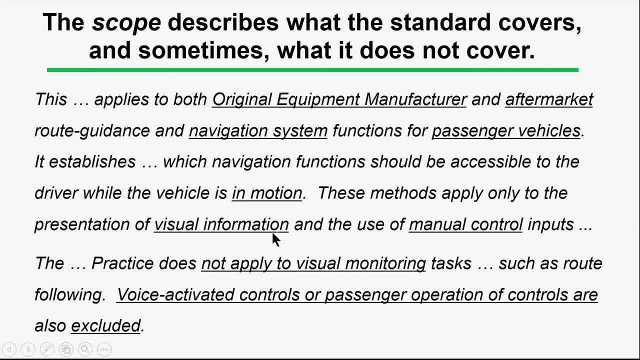 concerns than if you're actually driving. Another key point is that it only applies to visual information, so auditory information is not covered by this document and it only requires compliance with manual controls. so speech is not an issue, And there's some other issues as well. So the intent of the scope is to 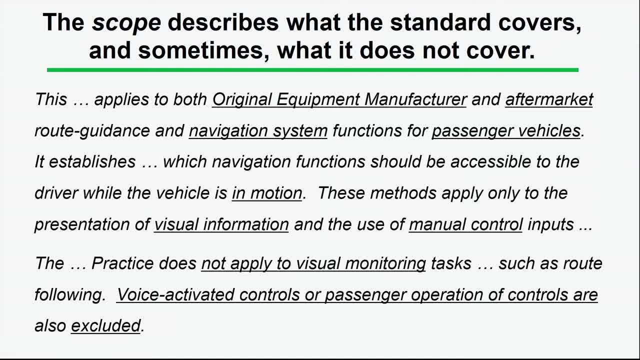 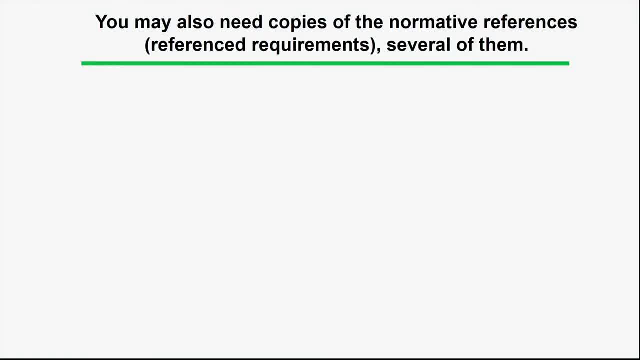 identify the coverage of the document. That is, what it covers and what it does not cover. In addition, documents have something in them called normative references. These are documents that are referred to and, because of the nature in which they're referred to, in some sense they are part of the standard and you 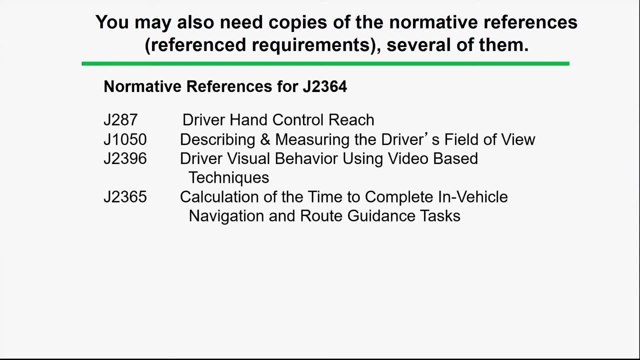 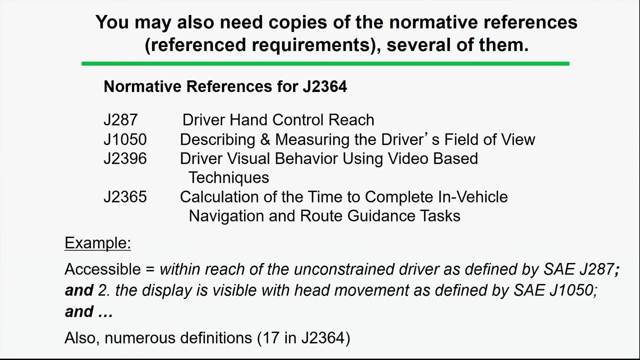 must have copies of them. So for J2364, as an example, there's a document on hand control, reach, field of view and some others, And here's an example of the text that describes or identifies why these normative references are so important. So, for example, the standard says that of interest is 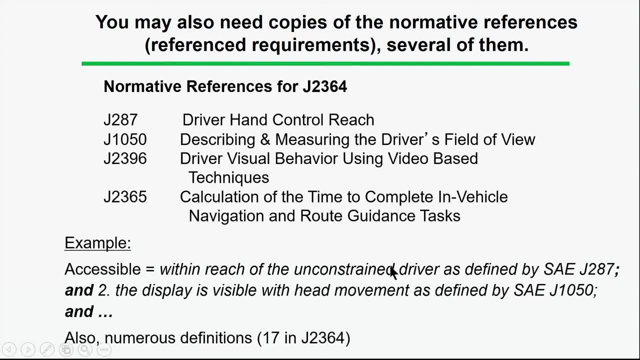 controls that are accessible. So what does accessible mean? Well, there's a definition in SAE J287, and also they have to be visible under certain circumstances, as defined by J1050.. So, therefore, to implement SAE J2364,, you also have to have copies. 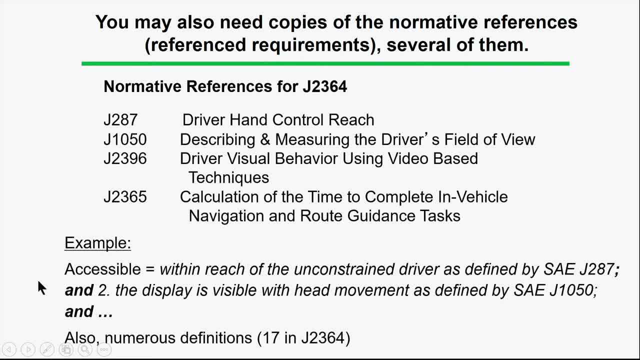 of J287 and J1050 to understand the document, And that's not unusual that in order to fully understand one standard, you often need copies of others, And in some cases it may be that the other standards have normative references and to understand them you need other. 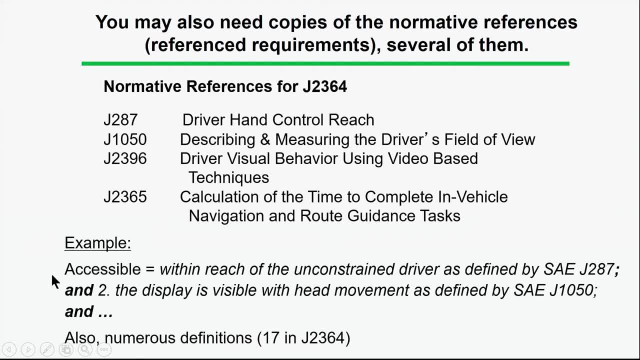 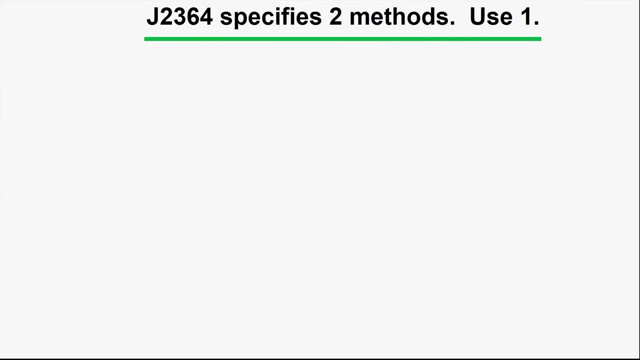 references as well. This is done because if all the information required to to understand the standard is in one document and pieces are changed in other standards, then multiple standards need to be changed and it's very difficult to manage the process. SAE J2364, because it 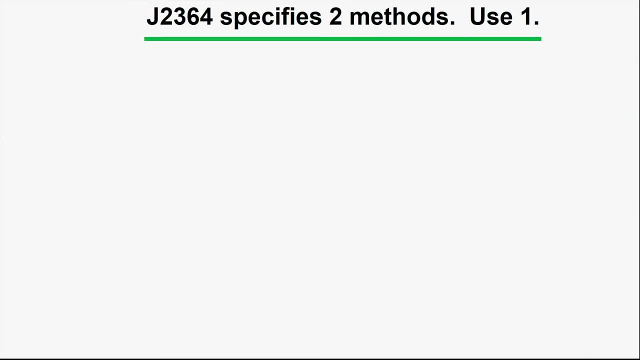 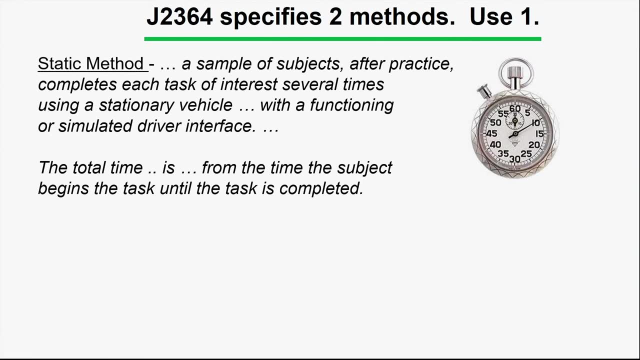 contains a method actually specifies two of them, And here's the two of them. So the first is called a static method, in which case people do a task and they're timed. how long it takes and whether it exceeds some deadline or not determines 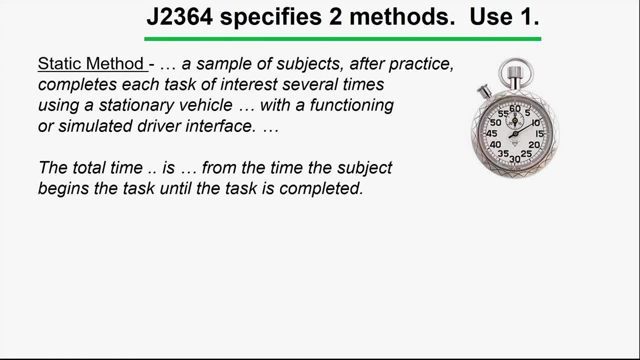 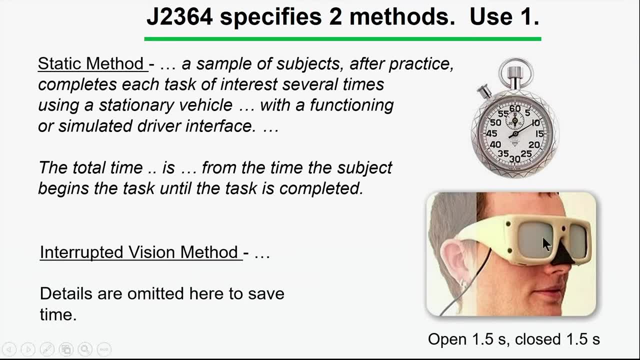 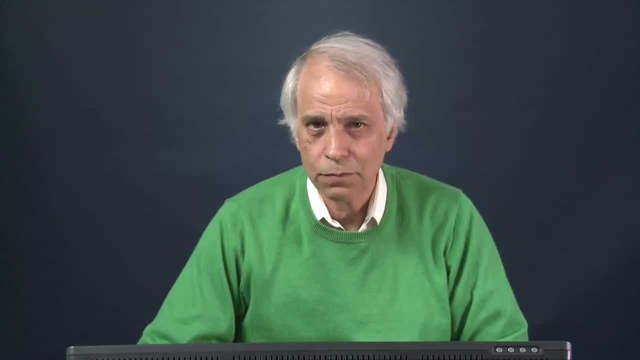 whether or not a task passes or does not pass some requirement. In addition, there's also a something called the interrupted vision method. So the subject wears a pair of goggles like this and they're asked to do some task. The goggles are open for a second and a half. 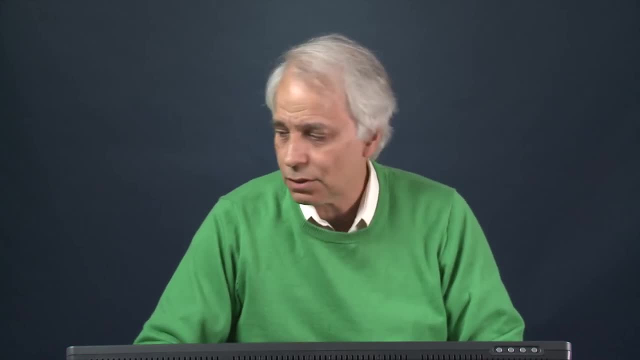 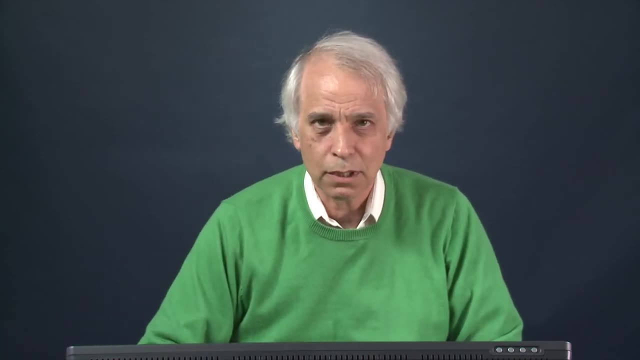 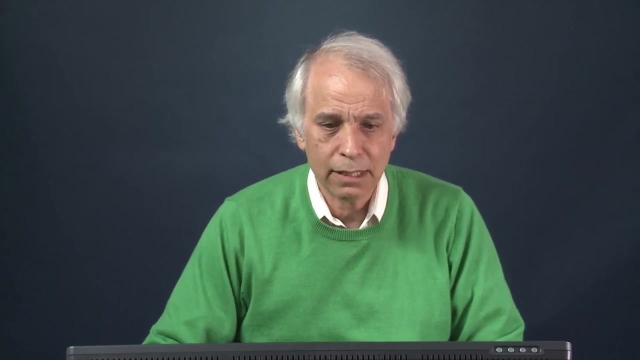 and closed for a second and a half. So that simulates the process of looking down and using the device and looking back to the road and looking down and looking down to the device and looking back to the road, with the closed period, correspond to when you're looking at the road. The details of the procedure are rather 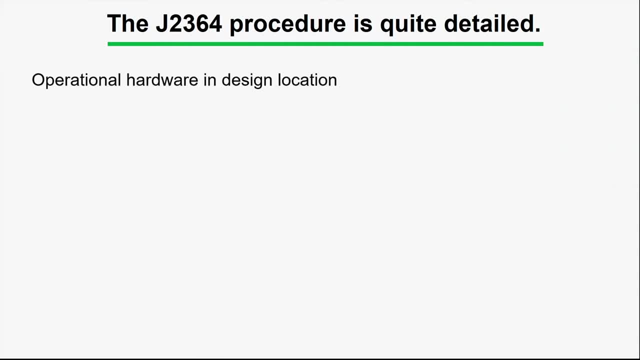 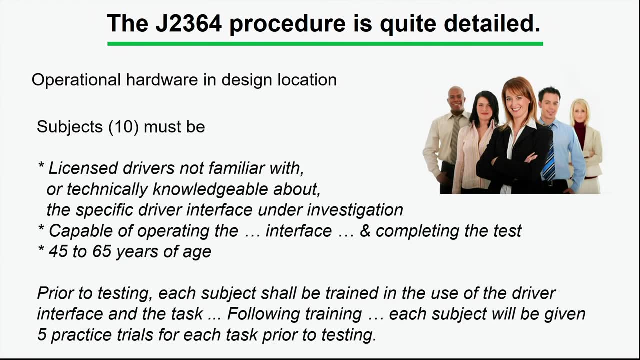 extensive and this is typical, again, of standards. So, for example, it talks about the requirement that the hardware be in the design location. There are ten subjects and there are a number of requirements for those ten subjects that they, in terms of their familiarity with the interface, that they can operate it. 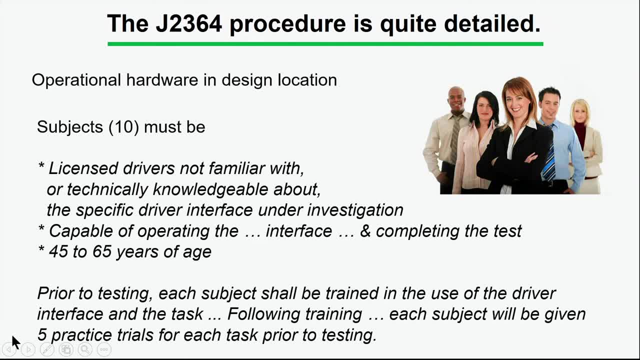 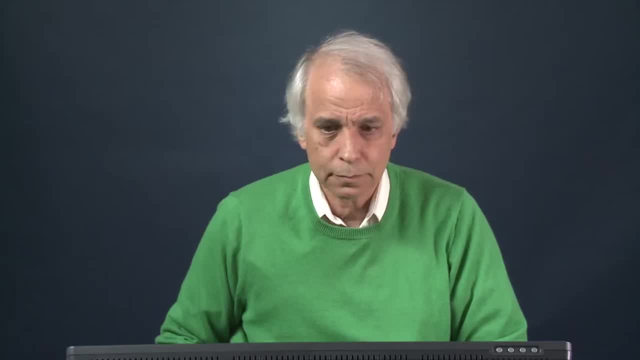 their age, their training, how many practice, trials and so forth- and this is pretty common for a good standard: that it has all the details, if there's a process involved, that describe how the testing is carried out, because you want the procedure to be replicable. In addition, this is an as somewhat unusual. 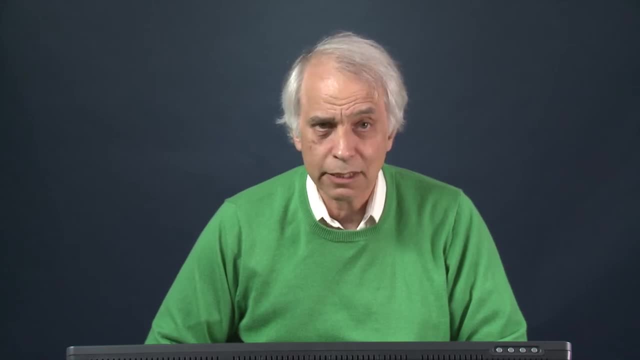 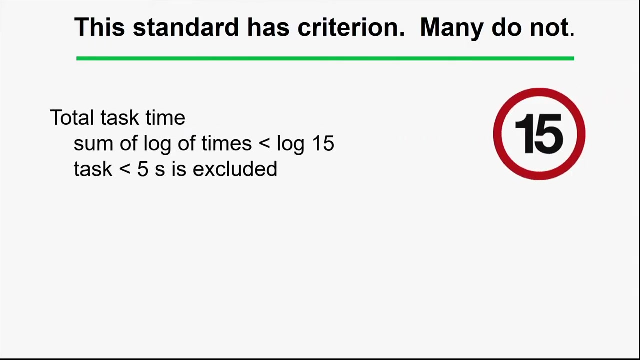 in that it has a performance criterion. Many methods documents just describe how to perform a test, but not what passes or fails, and in the case of the development of this document, there was a great deal of controversy about what should be the acceptance criteria. So in this case, for the static method, the total task time. 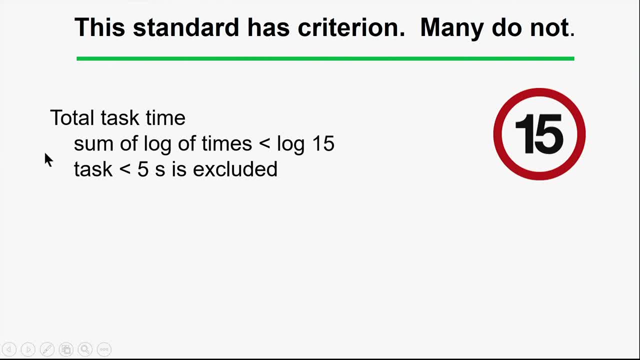 cannot exceed basically 15 seconds. It's a little more complicated than that because you actually take the log of the times and sum them and look if it's less than a log of 15.. This was done because some tasks had extremely long times on individual trials and adding them. 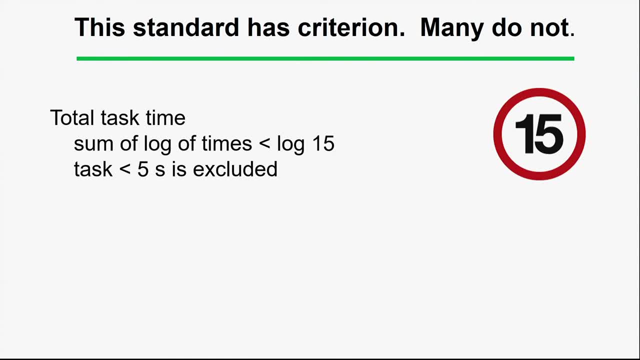 together in a strict, simple manner led to things passing when it was just kind of one oddball trial. that was, one was trying to eliminate And, in addition, if a task takes less than five seconds, it's excluded from the analysis. It just doesn't make any sense. It's just too short. Second is the 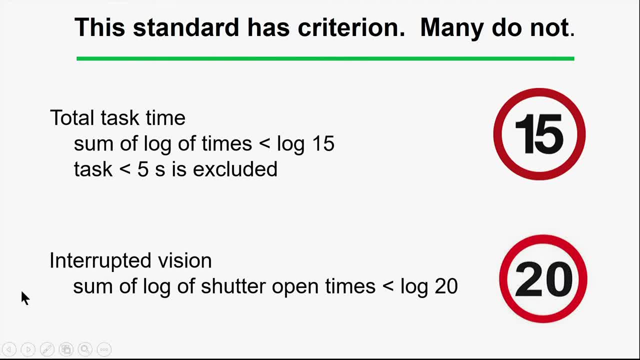 interrupted vision method and in this method we're looking at the times, the shutter, open times, and adding them up and then looking if they're less than 20 seconds. But again, it's a log procedure, not strictly additive. Again, to get rid of these, the 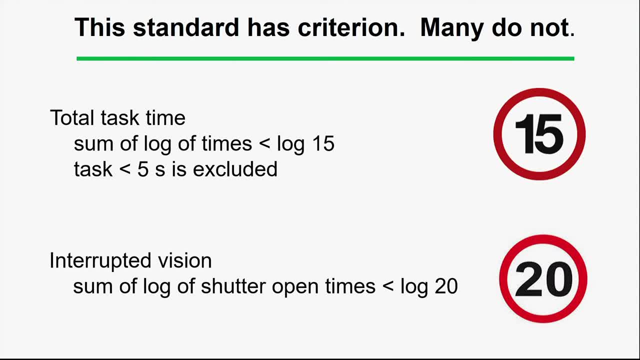 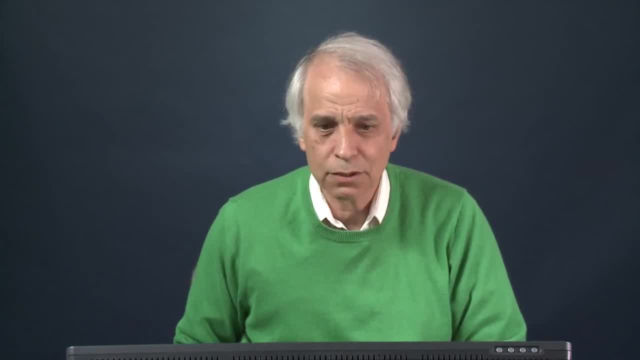 undesired effects of extremely long and rare trials. The next topic I'd like to cover is who develops standards in that and the process involved. The process is fairly consistent across many organizations In the United States government. they all follow the Administrative Procedures Act and 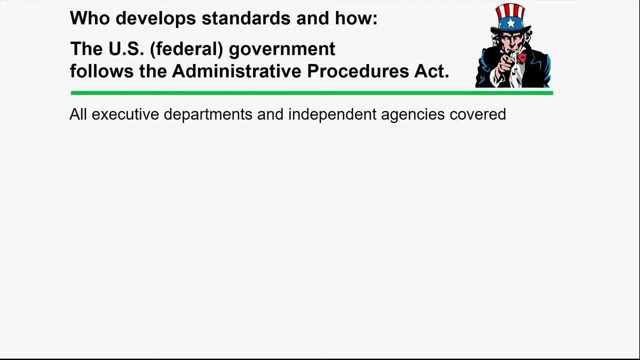 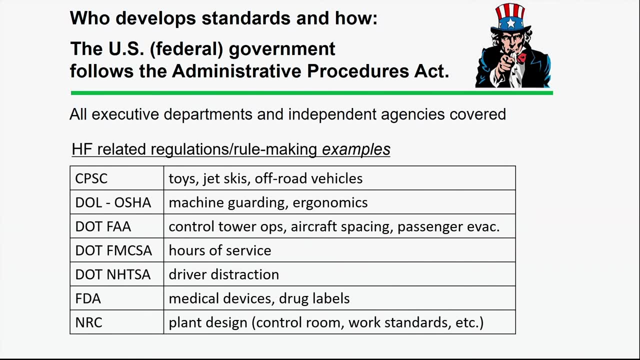 basically, a large number of organizations are involved that need to comply with this process, and here's just a quick list. So, for example, the Consumer Product Safety Commission is responsible for toys and jet skis and off-road vehicles. The Department of Labor is responsible for has issues. 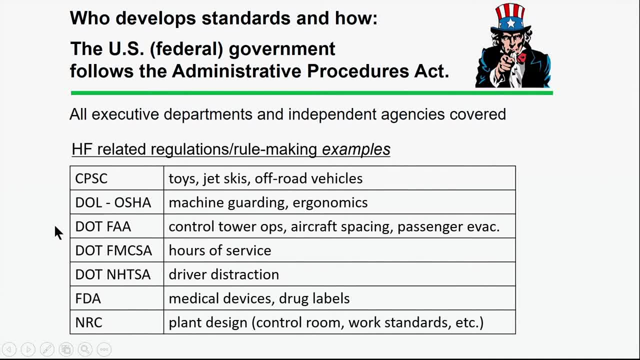 related to machine guarding that apply to human factors issues. The FAA: there are issues of passenger evacuation, all kinds of aircraft issues. The Federal Motor Carrier Safety Administration is worried about hours of service. NHTSA, the National Highway Traffic Safety Administration, is concerned with driver distraction. The 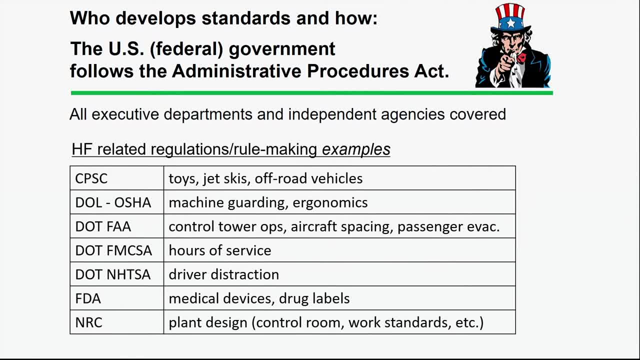 Food and Drug Administration is concerned with various kinds of medical devices, drug labels and so forth, And the NRC is obviously concerned with operation of nuclear power plants. So they they are also covered by this particular act. All of them have standards, guidelines and various other kinds of 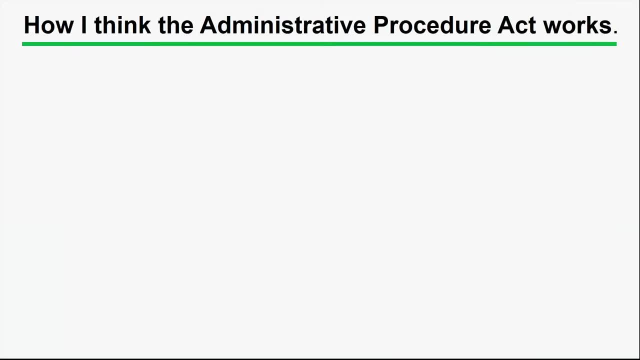 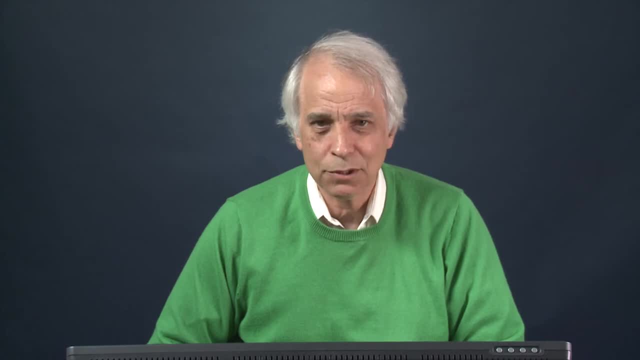 documents and they are developed following this particular method. So here's how it works. I'm not a lawyer so I'm not perfect in my description of it, but I think I can capture the gist of how it works, and I should comment that other organizations, like standards development organizations, follow the same basic idea. 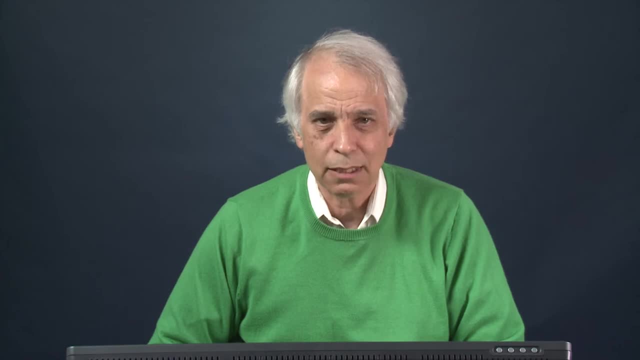 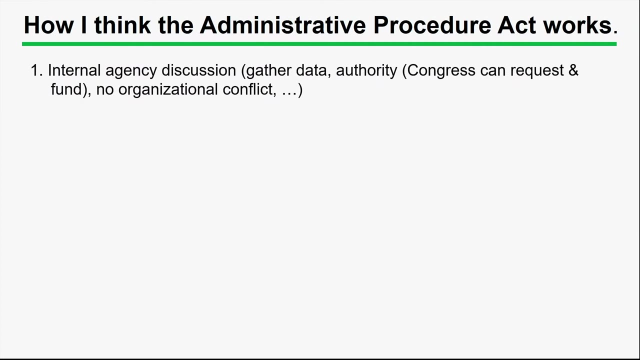 of making the process public and allowing for all parties to provide input. So the first thing that might happen is some agency within the government will say we need to have a standard on some particular issue. That may be the agency decides it's necessary or Congress passes a bill. 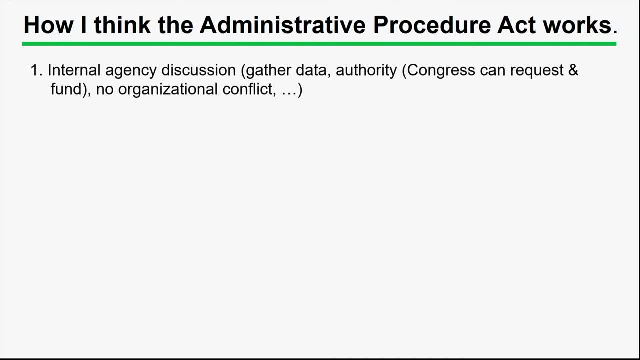 asking the agencies to act on some particular problem. The next thing that happens is that a document called a notice of proposed rulemaking appears in the Federal Register. The Federal Register is a document which comes out daily, which has print in it the size of an old-style telephone book. 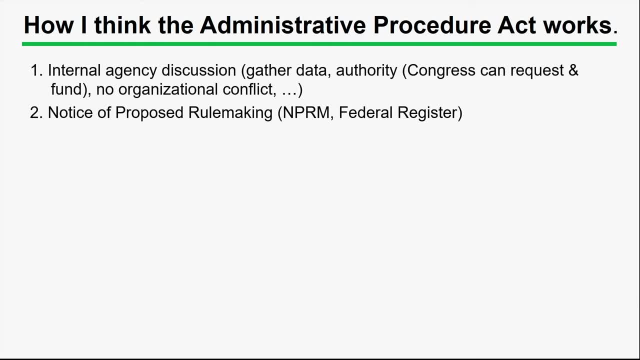 and often hundreds of pages, and it describes all the activities of the government for one day. So that notice appears in the Federal Register Looks like this: Then organizations are asked to provide comments on what the proposed rule or requirement is. That can be companies it. 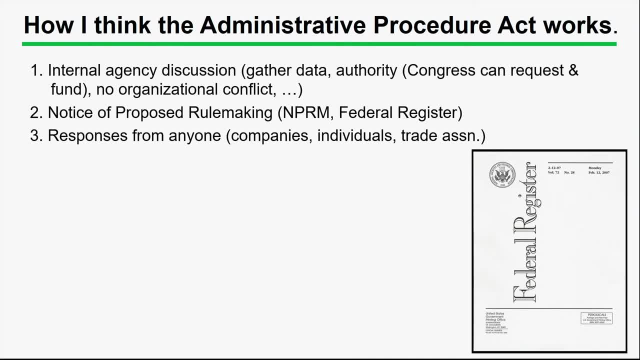 can be individual citizens who are interested in some topic and get wind of it. it can be trade associations, it could be unions, it could be any one or number of individual organizations or groups. There's no constraints on who's allowed to comment. The next thing. 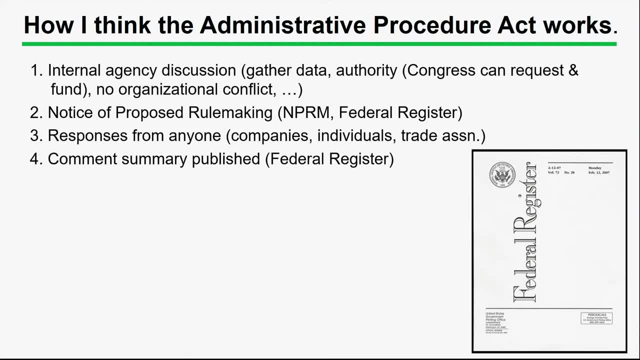 that happens is the government, after the comment period has ended, then takes all those comments and tries to provide a summary of how people responded And, surprisingly, even if an individual comments that person's name and sort of the gist of their comment and the government response to it can appear in. 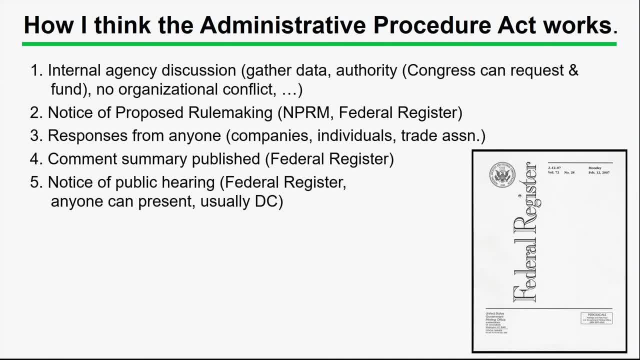 the Federal Register. Next thing that happens sometimes before this, sometimes overlapping with it, is a public hearing on whatever the particular issue is. Typically that's held in Washington DC because that's where the capital is, But it's not unusual if it's a major question for them to for there. 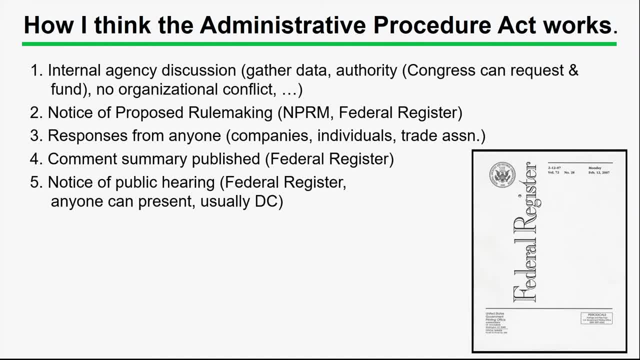 to be satellite hearings spread out across the nation. So there might be, for example, a hearing in San Francisco and one in Chicago. Or if it's automotive related, it might be in Chicago, Detroit, because that's where so many people related to automotive are. They try to make 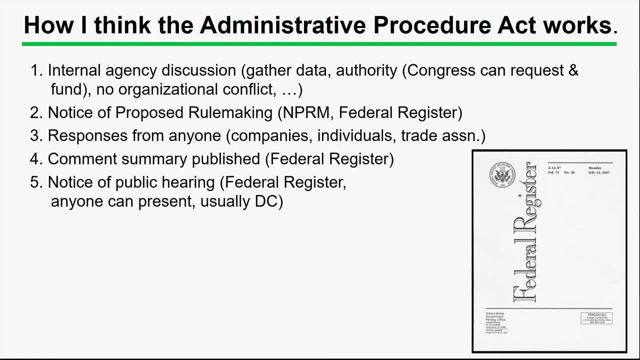 it in multiple locations and at least to give the public an opportunity to comment. It's very important in this process. Then, based on comments, the proposed rule is modified, There'll be some additional feedback provided based on the public input And eventually, 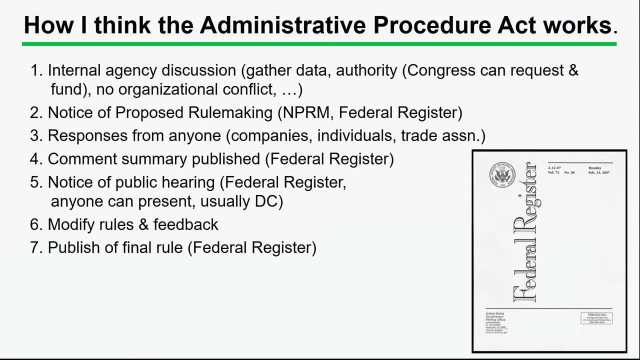 if indeed there's solid justification for it, that particular rule is again published in the Federal Register and it becomes the law of the land. It's not unusual in this litigious environment for there to be legal action contesting one part of proposed rules or another, And so it may take some time before the final regulation settles out. And my point 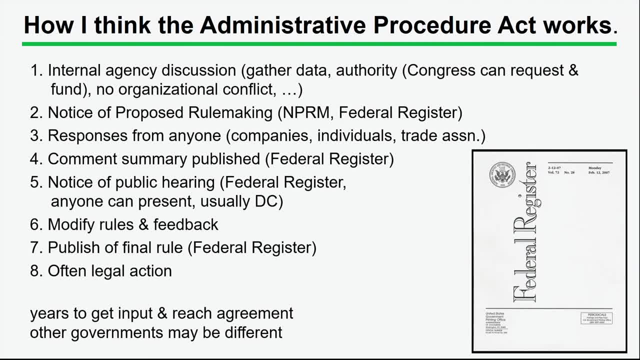 here is that it can sometimes take years to deal with that input And to get agreement as to how this process occurs. Other countries will have somewhat different processes, but the same basic themes are consistent across democratic governments: that they put something out to the public. There's opportunities for comment Those comments. 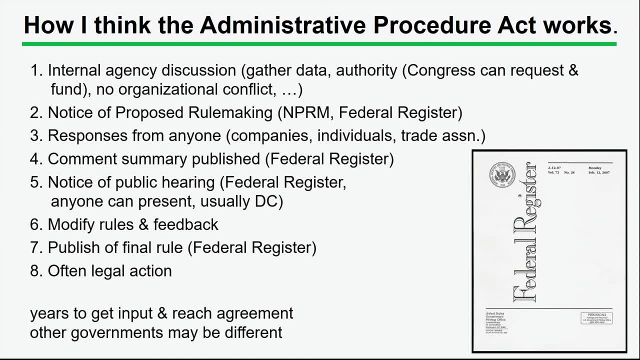 are considered. There's often specific replies to each comment. It doesn't mean the government's going to email you back, but there will be some public display of the comment, The kinds of comments that were made and how people responded to them, The regulations. 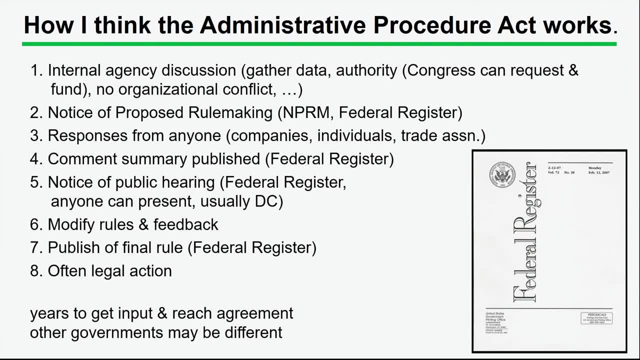 will be modified consistent with some of the comments. It doesn't mean that they always will be, but there's some serious effort to consider public input And then the item is published And again it's not unusual to have legal actions because some party's not. 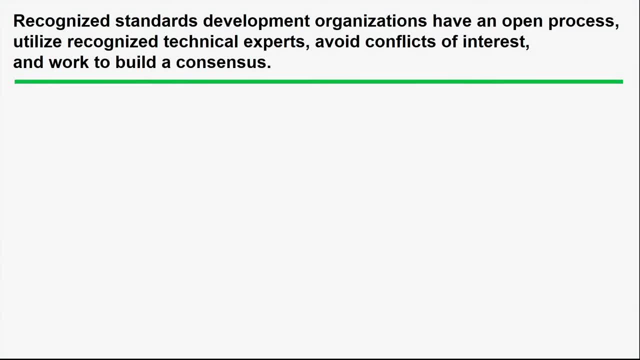 happy with the final decision. Standards development organizations other than governments basically follow the same process. Again, the key is to have, in this case, recognized technical experts. It's important that those experts have no conflicts of interest, And it's not a majority rule. It's an attempt to build consensus And so therefore it's important. 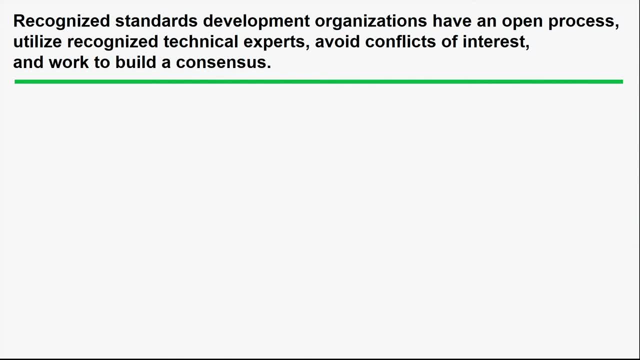 The need to build consensus takes time because you really want to get the parties to agree. That doesn't mean that everybody agrees to everything. But if an attempt is made within a standards development organization to get something to pass and only 51% of it are in favor, it probably will not move forward. It's going 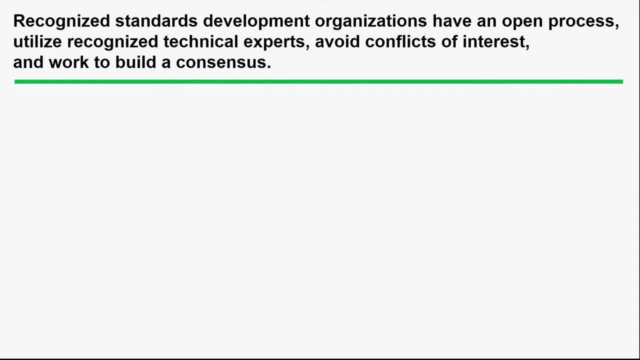 to take a real consensus, a real belief among a number of the experts that something should be done. This process is followed by professional organizations such as the Society of Automotive Engineers, the American Society for Mechanical Engineers, IEEE and so forth, And they develop the 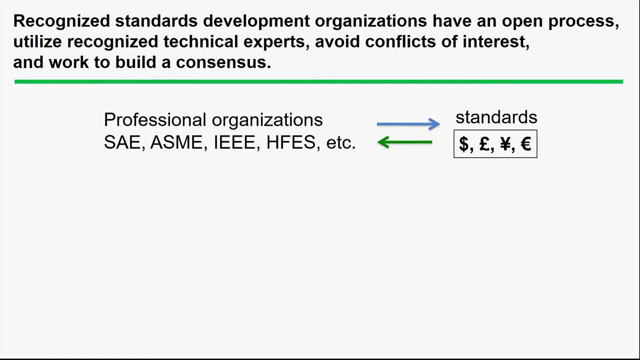 standards and other kinds of guidance documents. If an individual wants those standards, they need to pay for them, because it's payment for standards and other sources of revenue that allows these organizations to have standards development efforts. In most cases, that means publishing the documents, editing the documents, having a staff who goes to the various meetings. 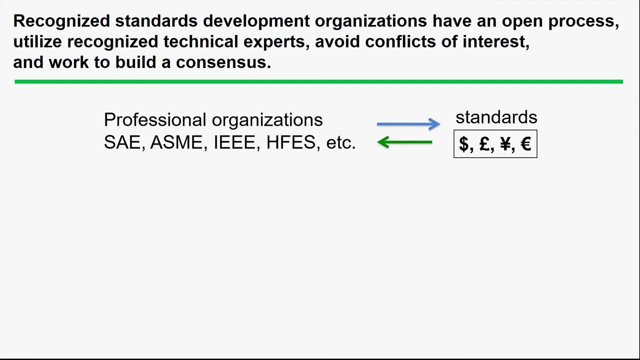 and takes notes who circulates the documents. It's a not it's not a trivial process in terms of expense. Those organizations, either directly or indirectly, will report often to national standards organizations. So for example, in the United States that's the American National Standards Institute. 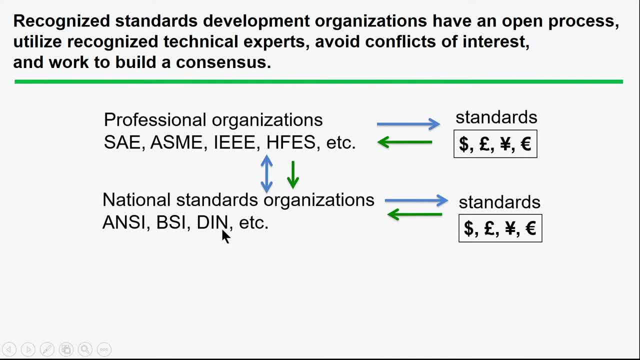 In the UK that's the British Standards Institute, In Germany there's an organization and so forth, And those organizations likewise support standards development efforts. Their efforts are funded by, typically, the sale of standards. These organizations can then report either directly or indirectly to international standards. 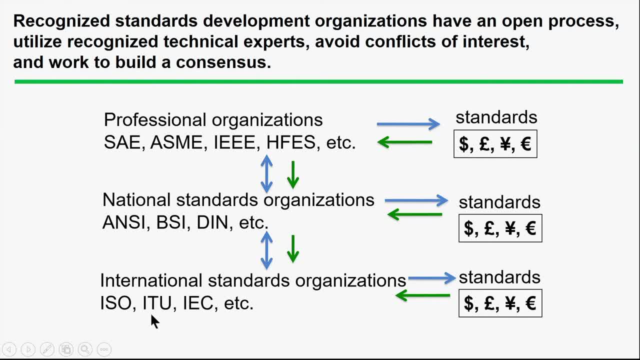 organizations such as ISO, the International Standards Organization, the International Telecommunications Union, the International Electrotechnical Commission and others. Again, these organizations sell standards as well, And so sometimes it's technical organization to ISO, Sometimes it's direct, Sometimes they're not. These two organizations aren't. 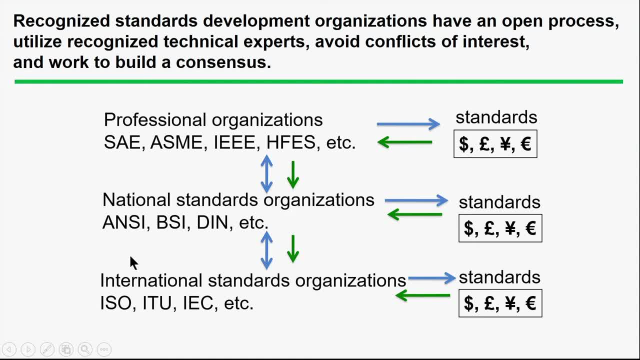 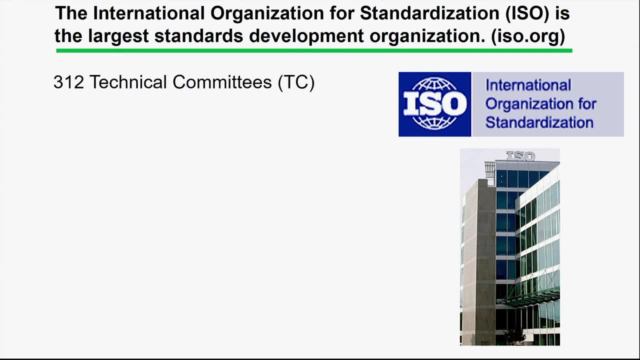 involved. It's just the national organizations are sending representatives but the actual standard happens at the ISO level. It varies very much with the standard. The ISO is the largest organization in international standards. effort To give you a sense of their scope: the last time I looked they had 312 technical committees and that number continues. 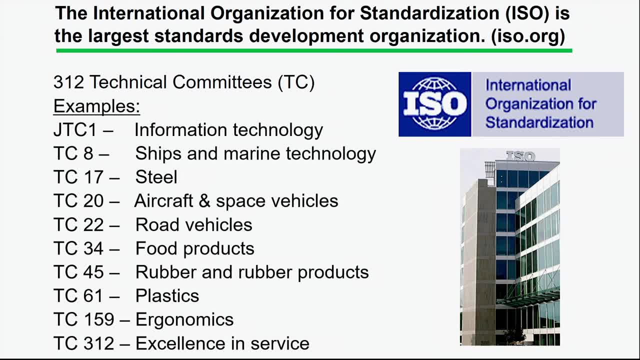 to grow. Here's some examples of some of the committees that exist to give you a sense of their scope. So one of the first ones formed was one for information technology. This is a joint technical committee. Technical Committee 8 has to do with ships, steel, aircraft, 22 is road vehicles. 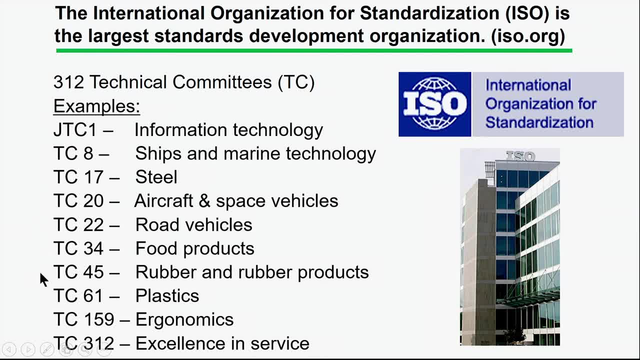 That's one that I'll talk about later- Food products, rubber and rubber products, plastics- Of interest to us is TC 159, ergonomics, And the last one that I noted down is TC 312, excellence and service. So the committees have gone over time from kind of fundamental technologies and fundamental 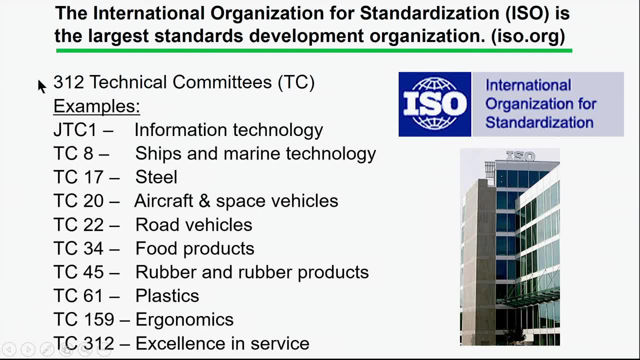 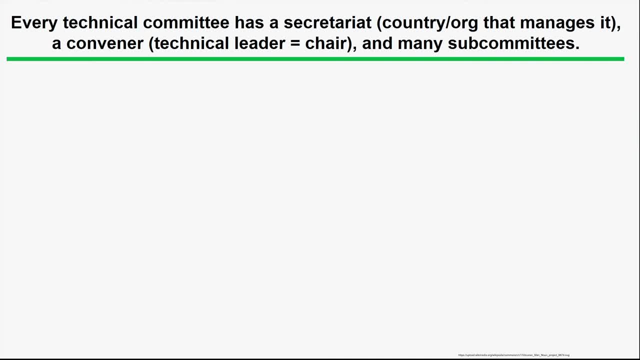 products more and more towards specialization as committees grow over time in terms of their number. The organization of a committee is as follows. First of all, every committee has a secretariat. The secretariat is the company, the country or the organization that manages it. So it 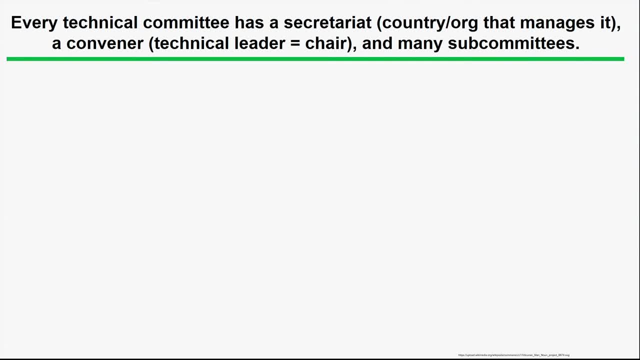 could be. the United States is responsible for something. The committee is led by a convener. That's the chair, the technical leader, And most committees have multiple subcommittees. So, as an example, Technical Committee 22 is, as I mentioned earlier, that's road vehicles. The country that's responsible for it is AFNOR. 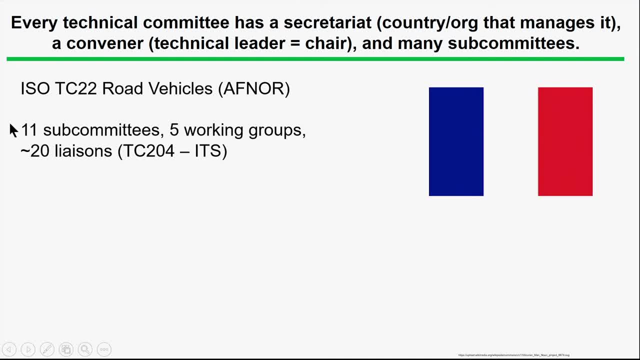 which is the French standards organization. That technical committee 22 has 11 subcommittees and five working groups And they're liaisons with other organizations and other committees because their activities, which for example vehicle technology, which is also the concern of TC 204.. So they need. 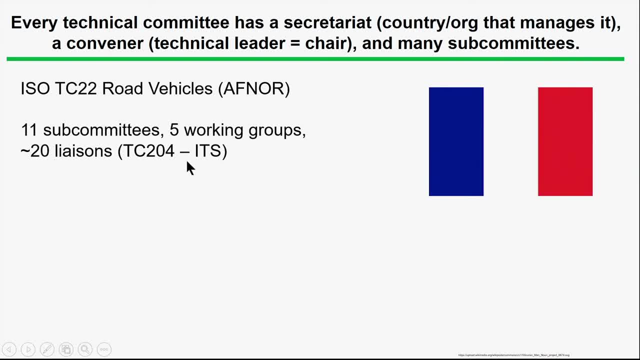 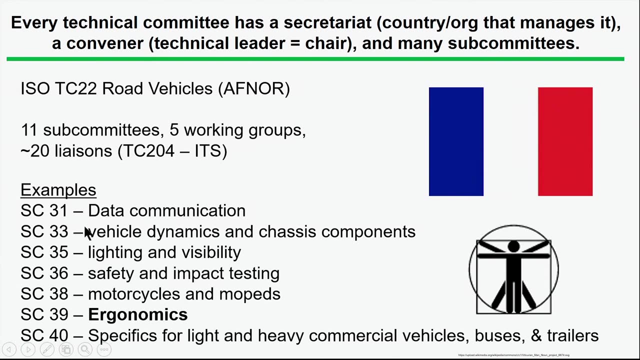 to know what the ergonomics people are doing, but the ergonomics people need to know what the technical, the vehicle developers, are doing, So there needs to be a liaison between the two of them. Here's some examples of some of the committees that are within Technical Committee 22. Data- 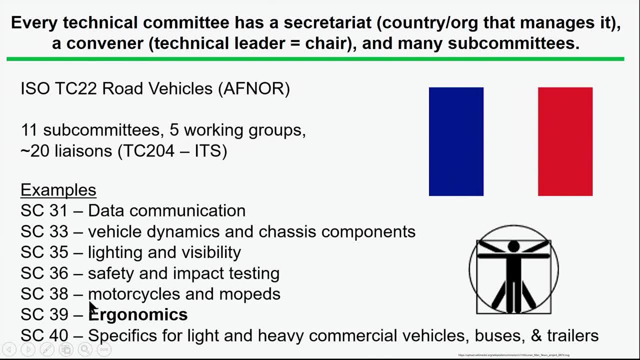 communication, vehicle dynamics, lighting safety, motorcycles are a special group, And obviously of interest to us is ergonomics, Subcommittee 39. And then, finally, there's also a special committee for commercial vehicles, buses, trailers, And it's not unusual to have 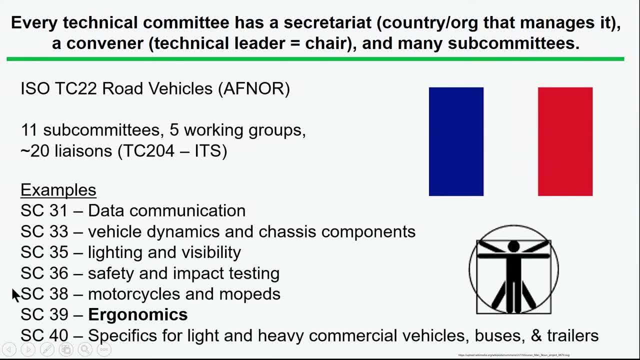 cars and light trucks being one group and sort of smaller personal vehicles being another, and heavy vehicles be a third subcommittee. You see that a great deal. So the next thing to mention are the subcommittees. So the next thing to mention are the subcommittees. 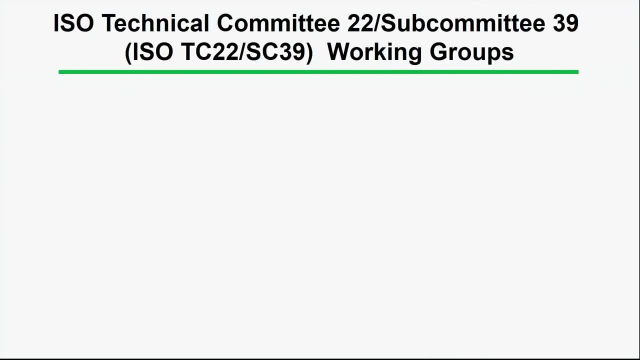 The next thing to mention are the subcommittees. So the next thing to mention are the subcommittees. These are the working groups associated with Subcommittee 39. Here's its official designation: TC 22,, SC 39. And here's part of the list. So there are four working groups: Control. 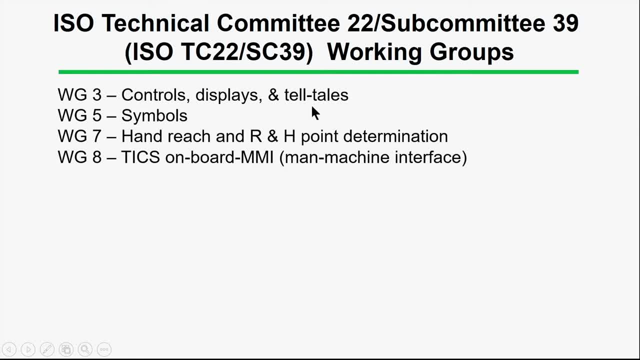 Symbols and Telltales. That's their technical name for warning lights, Symbols, Reach and Transport Information and Control Systems On Board, MMI Man-Machine Interface. Yes, there's lots of jargon. notice the committee numbers are not numbered sequentially. that's because has 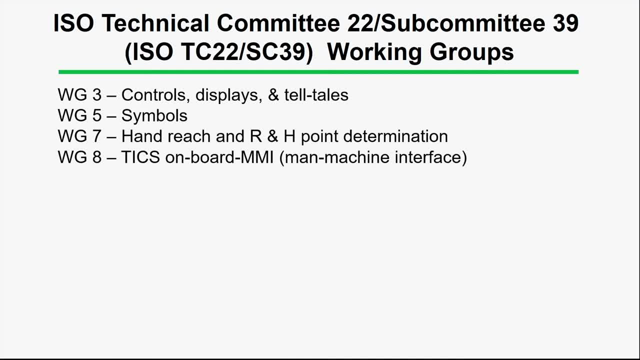 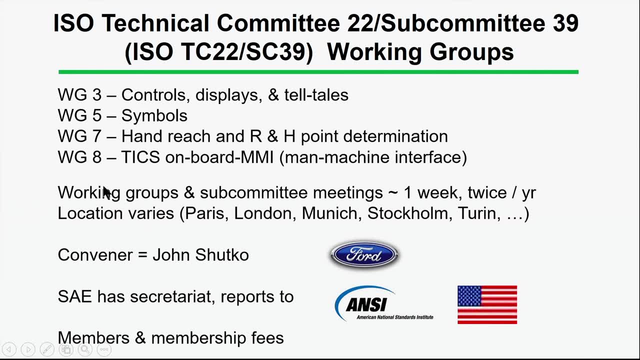 way back when other committees existed and they were dropped. in addition, these- this organ is. this subcommittee meets typically about twice a year. meetings are on the order of a week long and where they meet varies. often they meet in Europe, sometimes they meet in the United States and rarely they will meet. 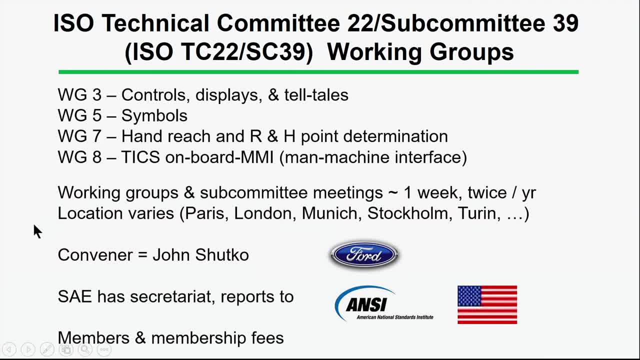 in Asia, sometimes in Japan, rarely in Australia. the main reason is because many of the members are from Europe. they want to minimize the average amount of airfare that people have to worry about, so unfortunately, the people in Asia often end up with bigger airfare bills than the Europeans or the Americans. one 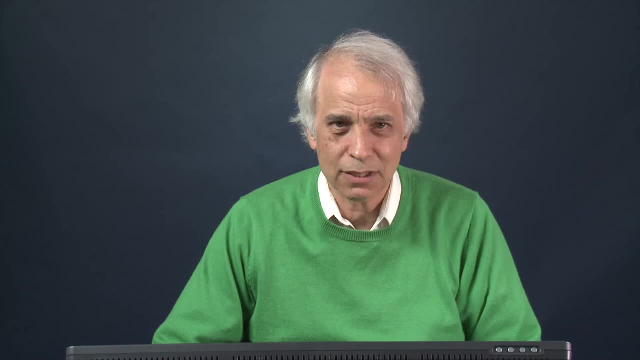 of the challenges is that people look at these activities and they kind of think of it as a boondoggle, because, oh, we're going to send this engineer to Paris for a week and the feeling is this is going to be just playtime and, quite frankly, the answer is no, they're going to be in. 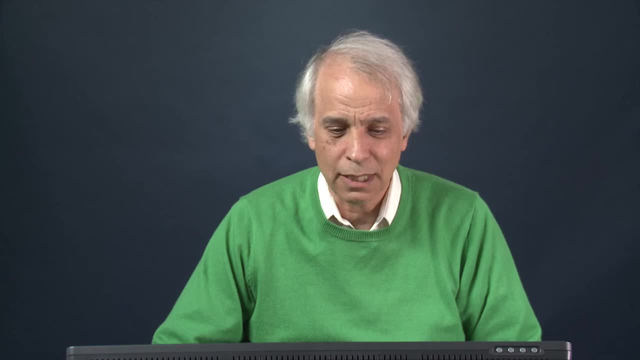 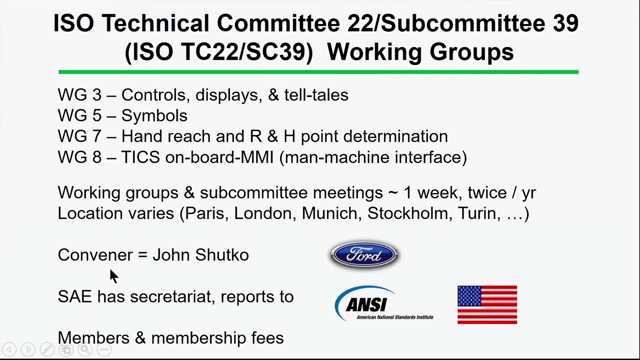 meetings pretty much all day. they may go out to dinner and have advantage of that, but they're not going to play tourist. the convener for subcommittee 39 is John Schutko at Ford the secretariat, the organization that is responsible for keeping track of the paperwork, for handling notes and meetings and so forth. 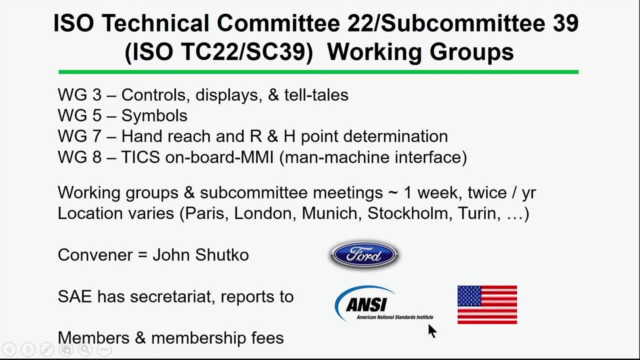 is the Society of Automotive Engineers. they report their activities to ANSI, which is the American National Standards Organization, now for the United States, and and to belong or to subcommittee 39 and to run it and to belong to ISO. the United States- actually ANSI, I believe- pays dues to the International Standards Organization. so not only do these, 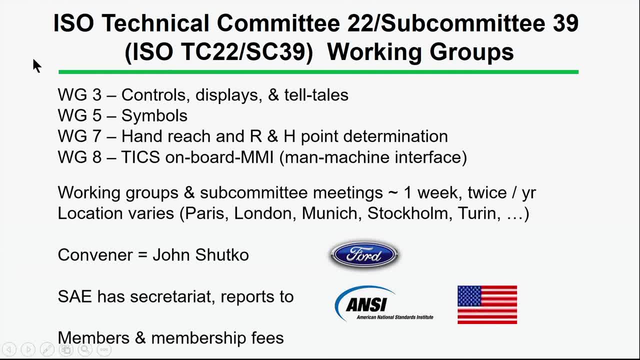 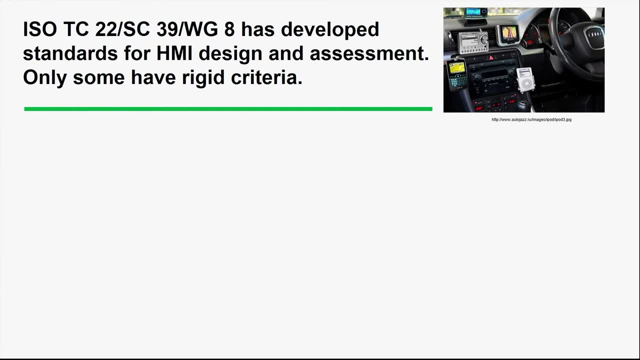 organizations need the sale of documents to survive, but they also need fees, membership fees from those who are participating in activities of ISO. I may have more to say about that later. so, um, the one that's of greatest interest to us is sub technical committee 22, road vehicles. subcommittee 39. 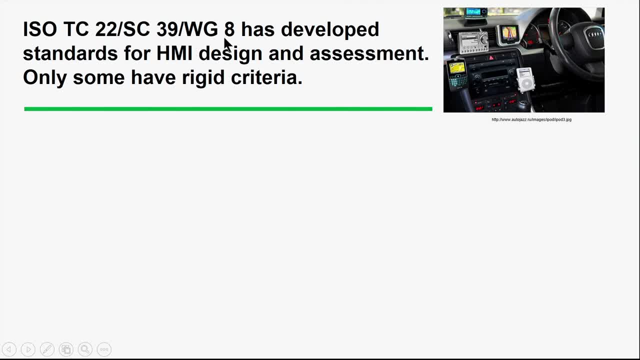 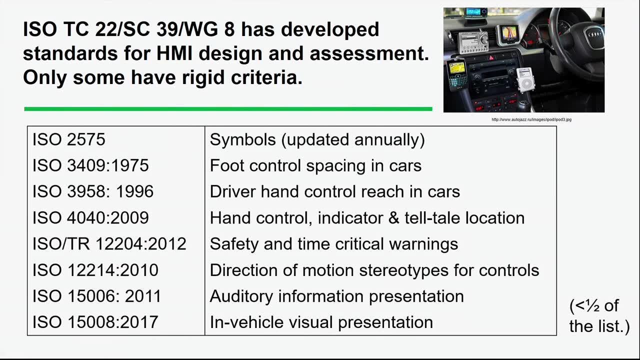 ergonomics working group 8, which has to do with technology inside vehicles. here's a list of of the standards that they have developed over time, and I just want to mention these to give you a sense of what they have done. So, for example, there's a standard associated with symbols- ISO 2575- that's updated every. 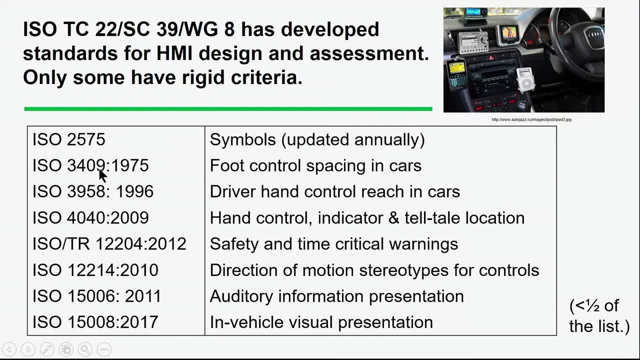 year. Every year there's a new amendment for some new standards that have been added. ISO 3409 has to do with foot control, spacing, 3958,, reach, and there's an SAE standard that's related to it. ISO 4040, where controls are located- 12204,. 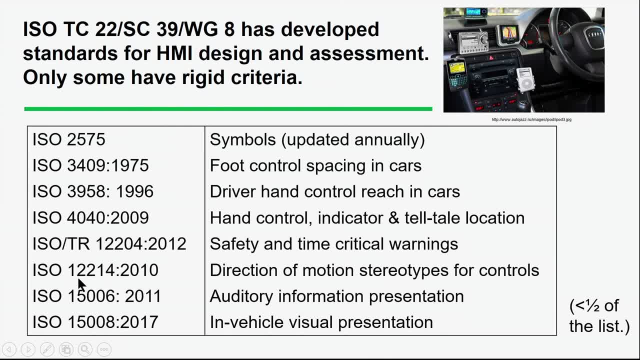 time. critical warnings 1224,. this one's been around for a while. direction of motion of stereotypes. If a person moves a control, how is the associated display expected to move? One on auditory information and then one on visual presentation of information, And again, this is about half of them that. 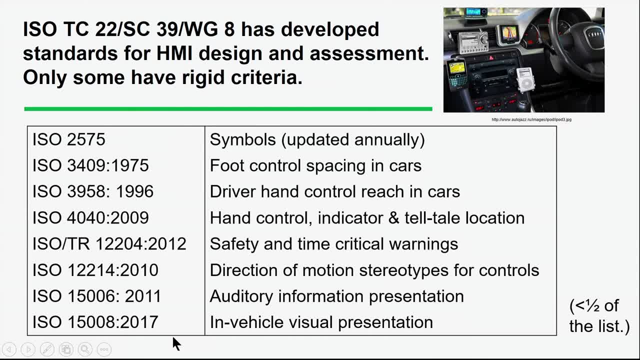 are out there. So I'm going to give you a little bit of an overview of the standards that they have developed. So I'm going to give you a little bit of an overview of the standards that they have developed. I'm just trying to give you a sense of what exists. So let me talk about the ISO. 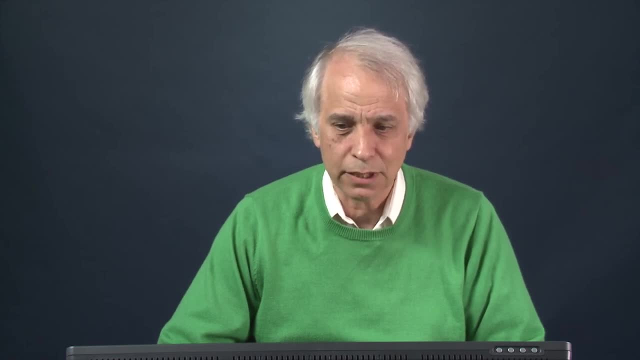 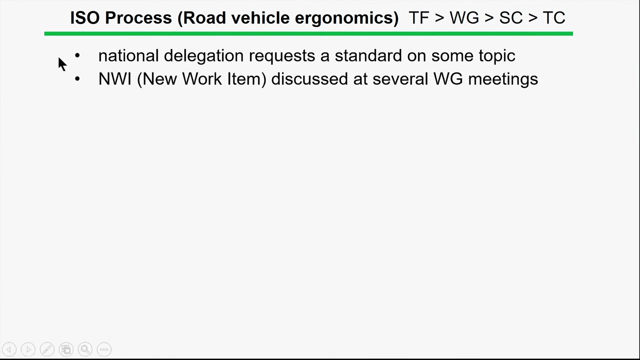 process which in many ways mirrors the federal process but is different, and you need to know some of the names of the groups and so forth are involved, should you ever decide to get involved in ISO activities. And so the process is something like this In an ISO unit, for example, Technical Committee 22,. 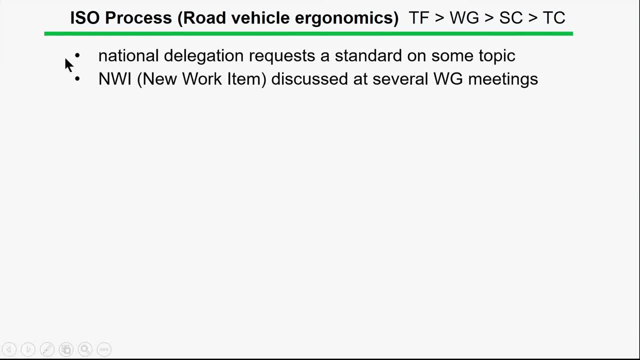 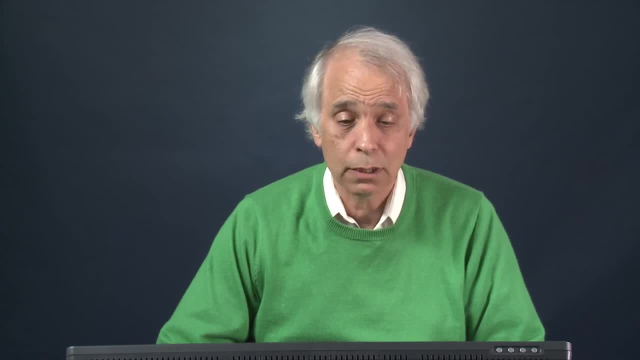 Subcommittee 39, one of the countries that has a national delegation requests some standard on some topic. So, for example, let's imagine that the automation work that's now becoming important was handled by Subcommittee 39. Then a delegation, say from Sweden, would say: well, we think there's a need for a standard on this. 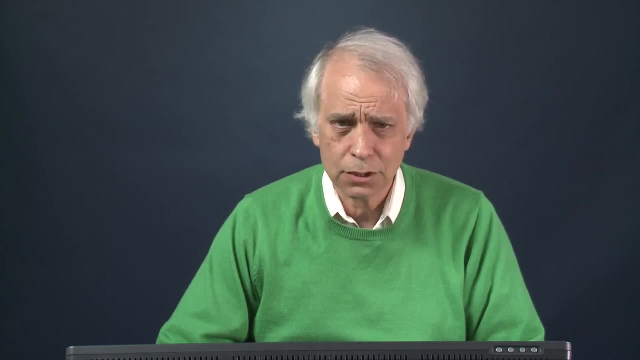 topic and here's some ideas about it, And that's usually discussed informally within the technical committees or subcommittees, usually for some period of time, And eventually it becomes what's called a new work item, meaning it's now formally on their agenda. 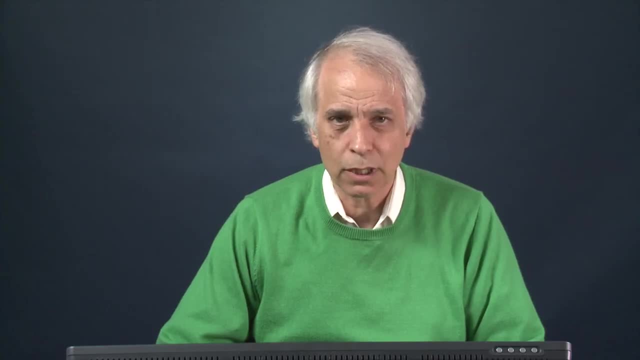 This is important because the time period from when a new work item is proposed and a standard must be published is three years, And if something does not appear in that three-year period after work starts, then it's discarded. So there's real pressure to spend some time to build a consensus. 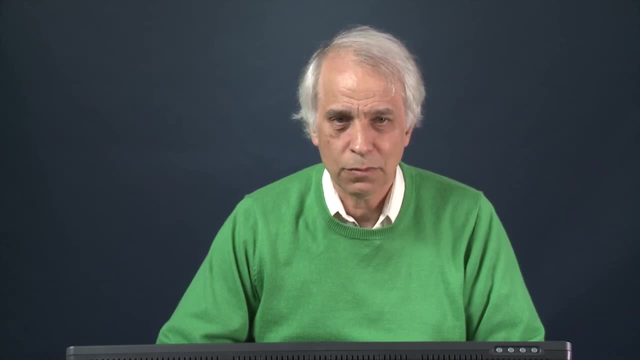 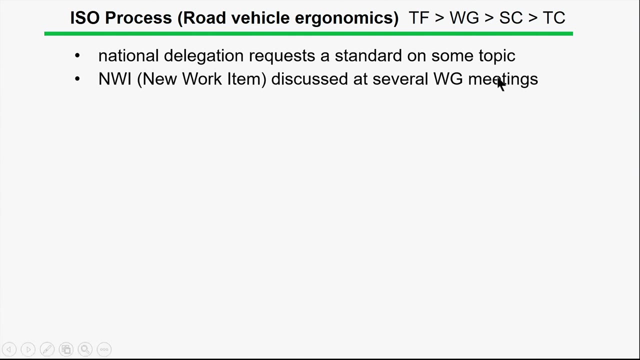 as to what's needed and to kind of do the groundwork before it becomes an important item, And so this is usually discussed, as noted, at the working group level. So the subcommittee has working groups and it's the working groups within the subcommittees where the real discussion happens and the details are worked out. 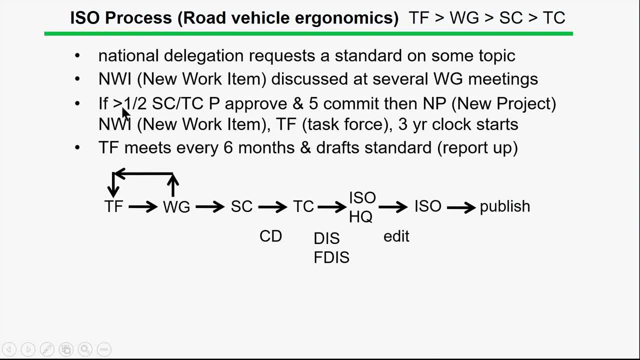 Now here's the actual specifics of the process shown in this figure. So the working group decides there should be a standard for some topic, or at least to consider it. That item is then identified to be associated with a task force which is a subcommittee or a subgroup of the task of the working group, And typically the. 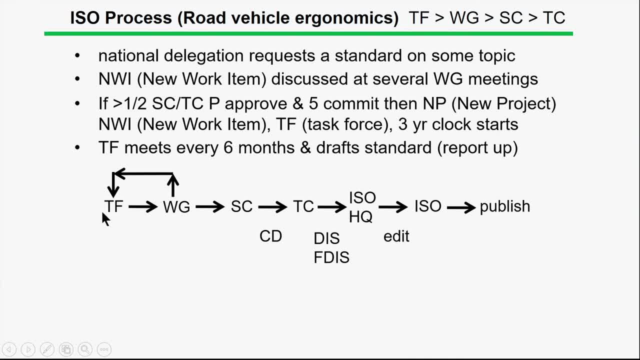 working group might be 10 people or 15 people. The task force might be 3,, 4, or 5.. It's just easier to get things done in a small group with the most interested parties, And there's a lot of back and forth between the working group and the 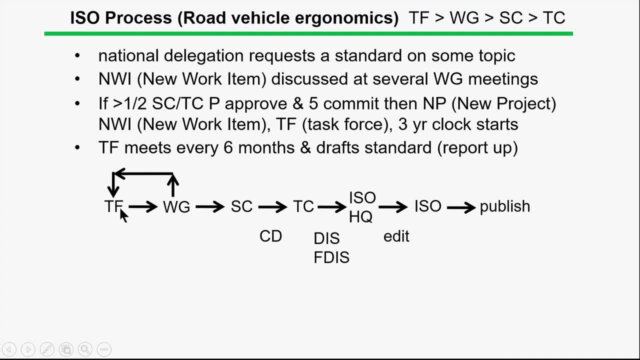 task force until there's real agreement as to what it should be, And I should comment that typically the task force members are just subgroup of the working group. There's not too many people on the task force who are not in the working group And the working 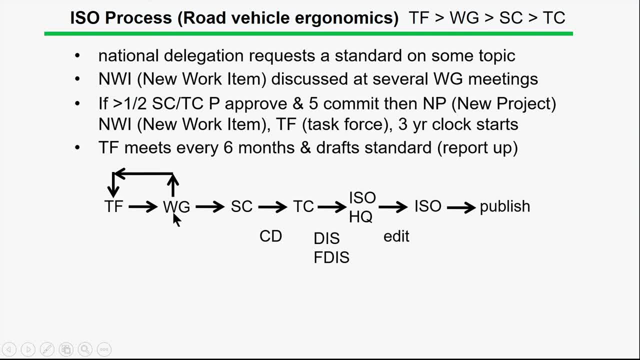 group is represented are representatives of people from a variety of countries, Most of those who are the major car producing countries: the United States, UK, Sweden, Netherlands, China, sometimes Korea, Japan and so forth. Now what happens is, once they have agreement as to what the working group is, 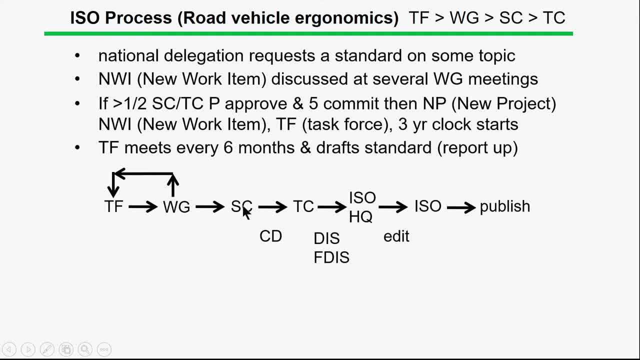 going what the standard is going to be at the working group level. then it's passed up to the subcommittee. Often a few members of the working group are members of the subcommittee, if not many of them, but the subcommittee consists of. 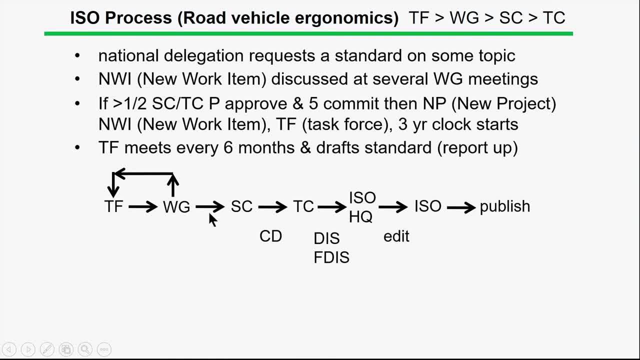 people from a larger group, from a larger number of countries, And then they'll debate the item and if they can say, we agree with it, in which case it becomes a committee draft that's passed along to the technical committee, The next level up- or they can be unhappy with once developed have 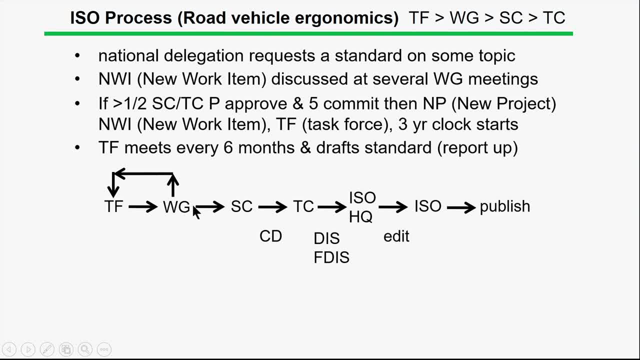 questions, comments and it gets passed back to the working group. I should comment that, as the working group is doing their tasks, they're giving reports to the subcommittee, so the subcommittee has a heads up as to what's going to happen. So it goes to a committee drafted. subcommittee has to vote: working group. 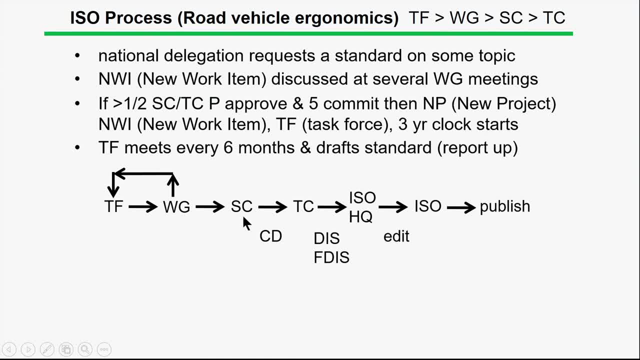 votes are by individual subcommittee votes start to become votes by country. technical committee votes are always votes by country. So when you're at the technical committee level it's very much like the UN, where each country has only one vote. Then, if the technical committee approves, it becomes a draft international standards. 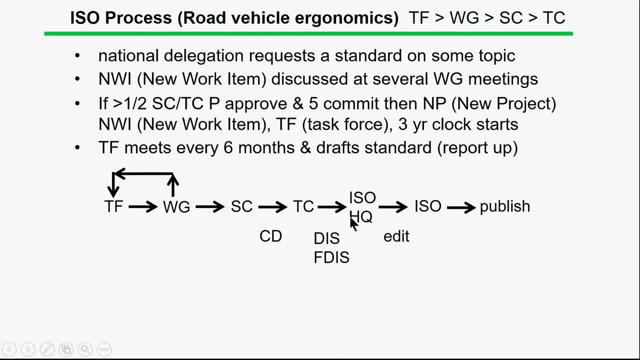 and then a future draft international standard. It's passed along to the ISO headquarters in Geneva. They do editing. They make sure the translation into French, if it was developed in English, is appropriate. There's always some editing. It then goes along to the main ISO unit and it's published. 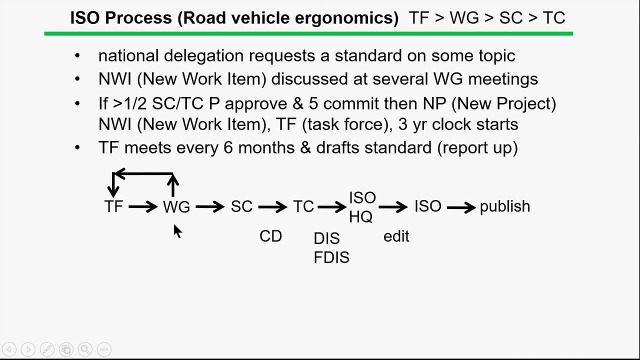 And again, this process takes several years to accomplish, But the goal is to develop a document for which there's consensus support that's based on solid evidence that countries all over the world will adopt. That takes time. Comments about the delegates, because I think this is important. 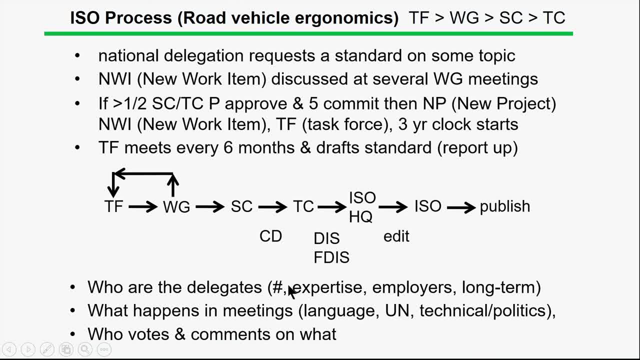 Each country has sometimes not too many constraints in the number of delegates you can send to a working group. Clearly you don't want too many, because it's just not effective And the problem is funding these individuals. So, for example, typically these are individuals who either represent their governments or 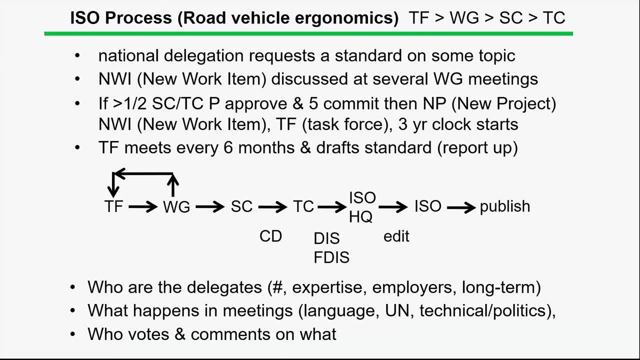 represent companies, because companies see that there's an important interest in developing international standard and they want to make sure that their processes, their products and their services are compliant. It's usually the case that they have some expertise of the topic. The amount of expertise varies. 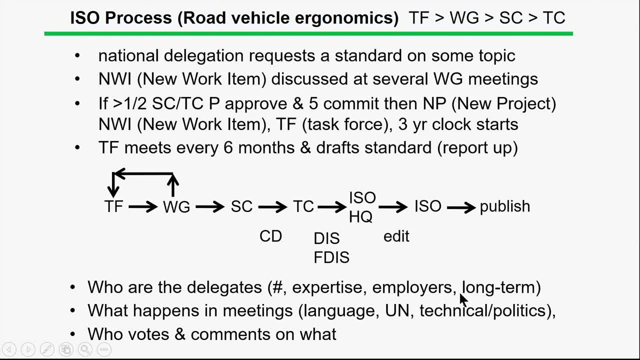 People who do serve on these committees invariably have to make a long-term commitment, And my experience has been that if you come in and think you're going to be on a committee for just a year and leave, you're not going to be very effective. that it's usually after.